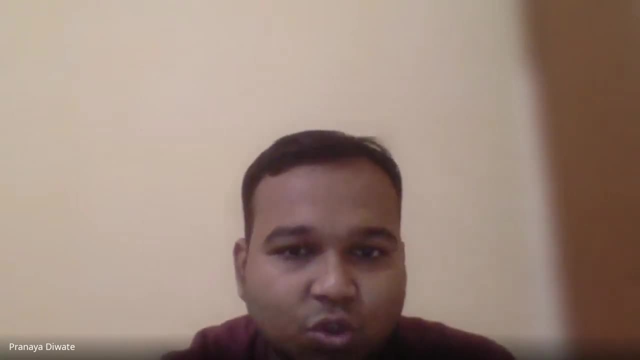 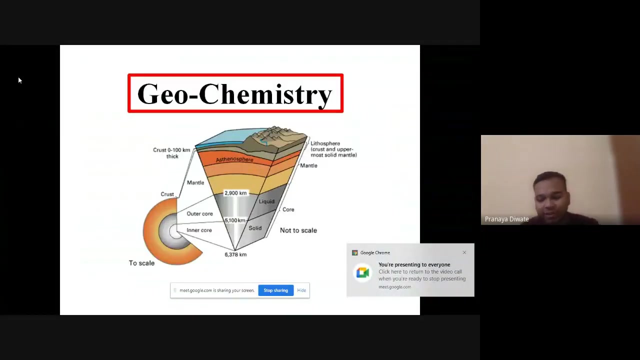 is involved: the geochemistry component. Without geochemistry you are not going to go more ahead with the specific physical properties and all. So you need a chemical property of that particular rocks or mineral, whatever you are looking for, to see that what kind of material are they built with? So the what we are going to now, the what is geochemistry. 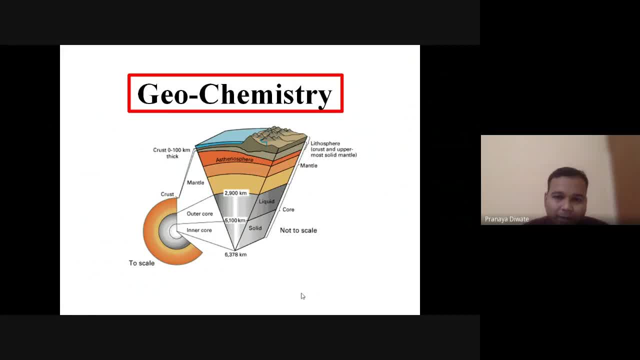 So geochemistry means earth, chemistry means what we know about the chemical science. So geochemistry is the study of the earth, So chemistry of the earth. basically, our earth is divided into the different layer. That layer is basically mental and core. We divided our earth into three different layer, that is crust, mental and core. After the this: 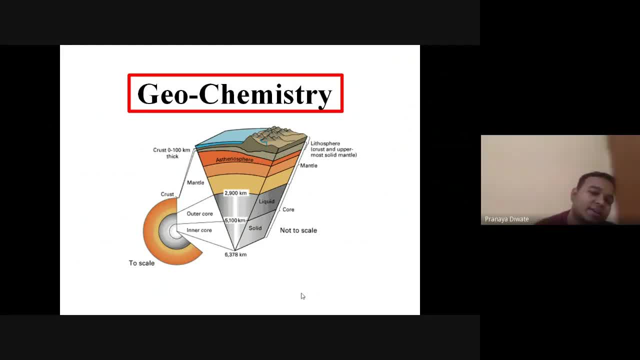 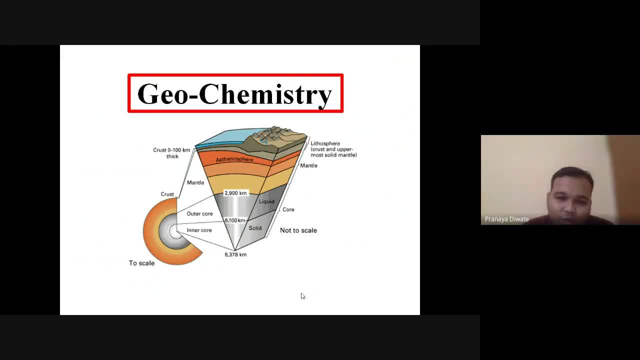 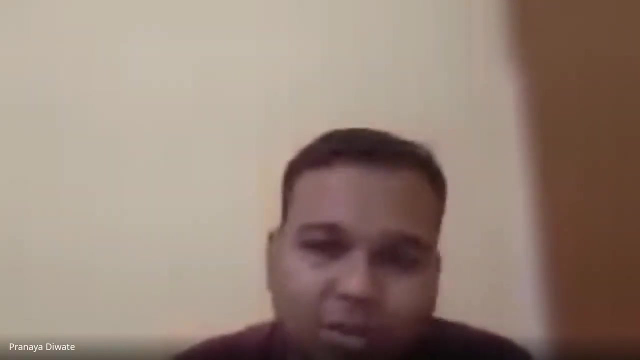 So also its a central with a C-R cycle Malai structure. So basically you have a in earth. so itself you have a different type of chemical composition built in. So for that purpose generally you should know about the geochemical composition of the earth. 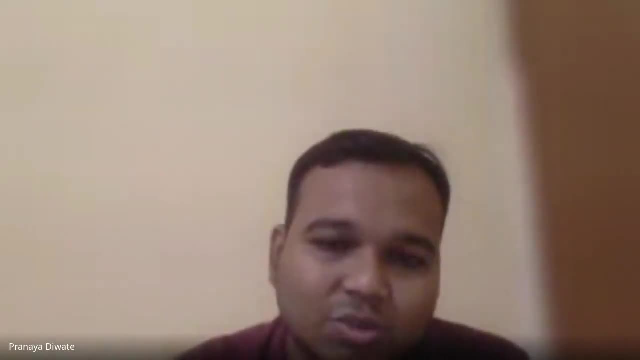 What kind of strata you are looking for or what kind of strata you are looking for. So that is known as the geochemistry of the earth. So the geochemistry is the field of. the geochemistry is the field of involve the study of the chemical composition of earth and other planet. The study of chemical composition of the earth and other planet is study under the geochemistry. 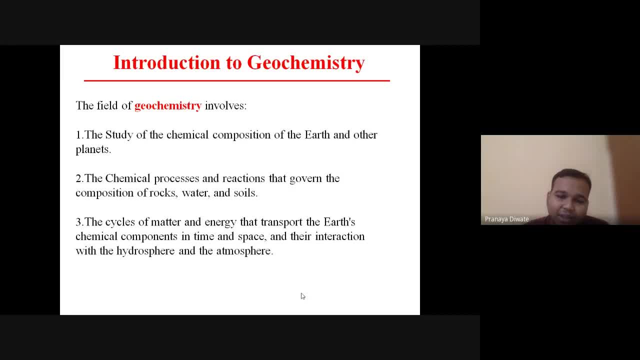 The chemical process and reaction: chemical process and reaction that govern the composition of rock, water and soil. So the geochemistry is the study of the chemical composition of the earth and other planet. The chemical process and reaction that govern the composition of rock, water and soil. The cycle of matters: cycle of matter and energy that transport the earth chemical component in time and space. 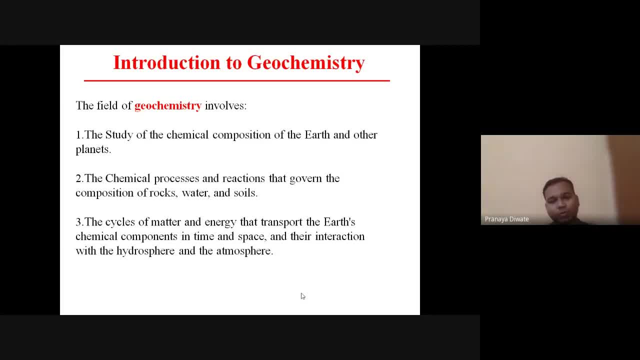 And their interaction with the hydrosphere and atmosphere. So the what the geochemistry is basically involve the study of chemical composition of earth and other planet. So geochemistry is not only limited to the earth, the other planet like mars, and all the, whatever the mission we are going to take in the various other planet. 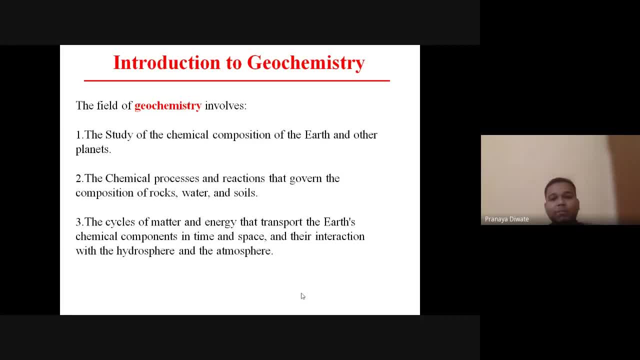 We are also going to see the what is the geochemistry of that particular planet. So the study of chemical composition of the earth and other planet is involved in geochemistry: The chemical process and reaction that govern the composition of rock, water and soil. 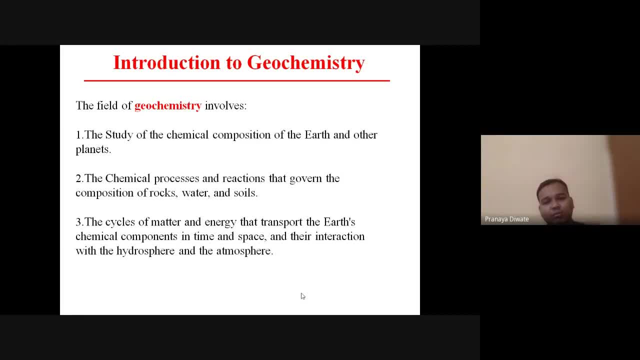 So the chemical process and reaction that govern the composition of rock, water and soil, Then the cycle of matter: the cycle of matter and energy that transport the earth chemical component in time and space, And their interaction with the hydrosphere and the atmosphere. 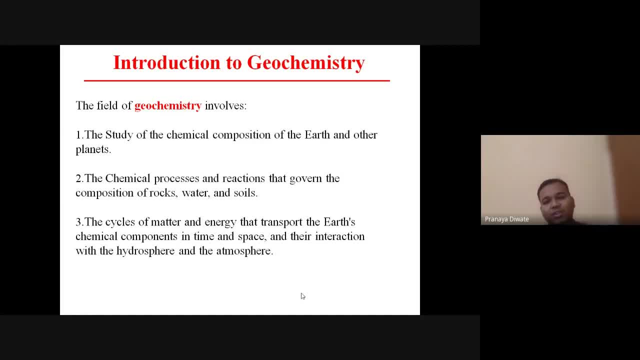 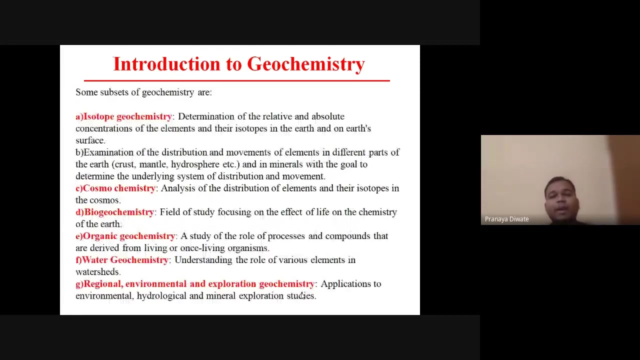 So the geochemistry, or chemical process reaction that governs the composition of rock, water and soil, The cycle of matter and energy that transports the earth chemical component in time and space and their interaction with the hydrosphere. So the geochemistry is a geochemistry also. you have a different kind of branches of geochemistry. You have a different kind of branches of geochemistry that having some different sub-branches also. 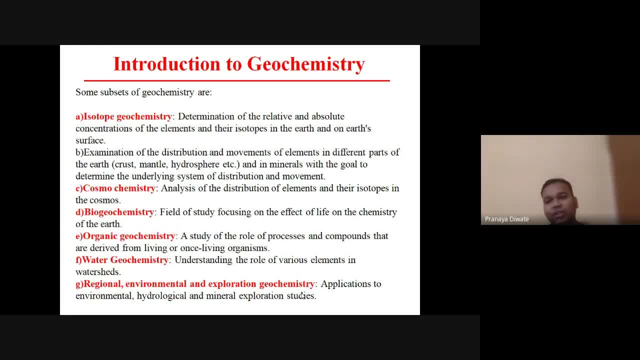 The geochemistry itself is a branch of geology under which you have several other branches. What is that? branches? which is that? branches? Isotope geochemistry, Isotope geochemistry of geochemistry, determination of the relative, determination of the relative absolute concentration of element and their isotope in the earth and on earth surface. so what, uh what? 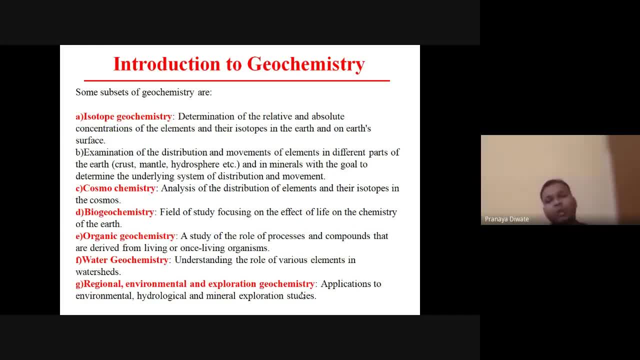 the isotope. geochemistry is all about the determination of the relative and absolute concentration of the element and their isotope in the earth. so, uh, what is the isotope actually? if you have a same mass number, different atomic number and all theories of chemistry, you already 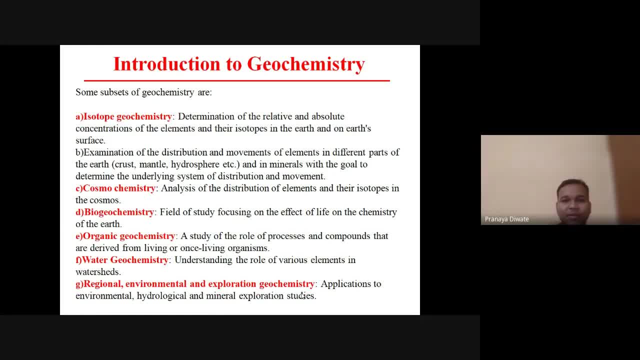 studied 12 here plus 2. what is isotope, what is isobar? so that all the concept is the same one. here you have a same atomic, different atomic number, same mass number and all. so that same concept is also applied here about the isotope. but when you study about the isotope, when you 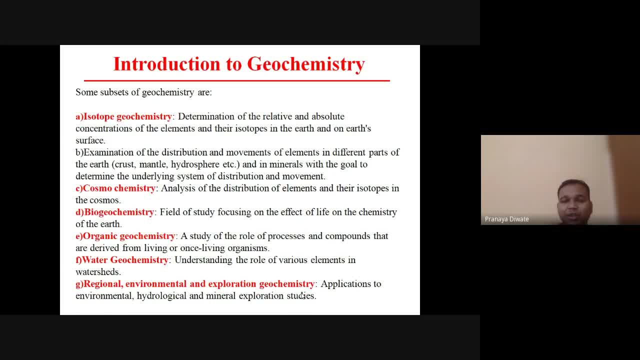 study about the isotope. you have some implication of that isotope. isotope is always been useful, or more useful, in geology for a determination of any uh strata, determination of relative absolute concentration of the element and so that we can come to know about the age of the. 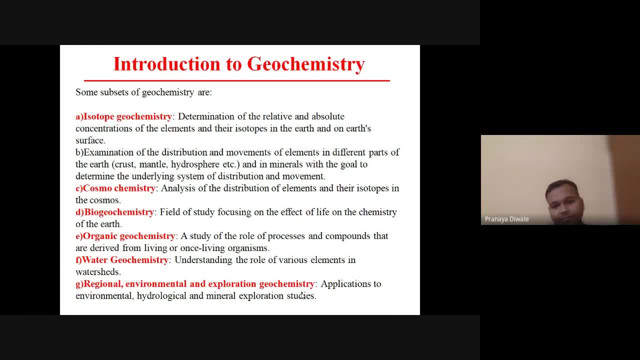 earth, you should come about the age of the earth. then you have a cosmic chemistry uh analysis of analysis of the distribution of element and their isotope, the cosmogые analysis of the distribution of element and their isotope in the cosmo. that is known as. 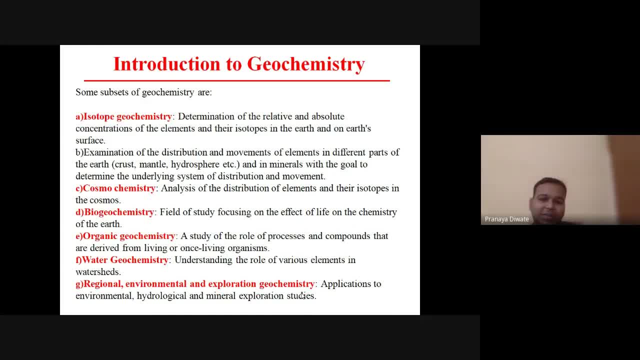 cosmic chemistry. then you have biogeochemistry, then you have biogeochemistry- the biogeochemistry- a field of study that is focusing on the effect of life on the chemistry of earth, the field of study that is focusing on the effect of life on the chemistry of the earth. then you have organic. 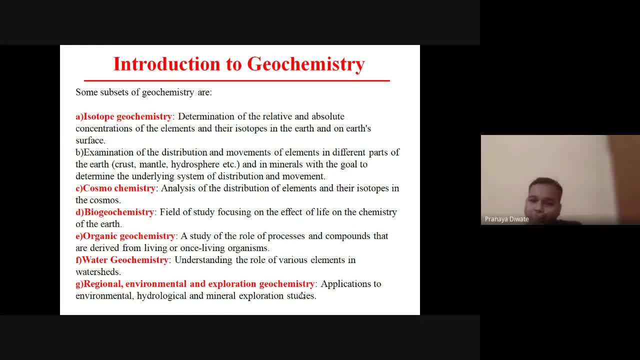 chemistry. then you have organic geochemistry. organic geochemistry is a study of the role of process, study of role of process and compound data derived from the living on or once living organism. a biogeochemistry is a field of study focusing on the effect of life on the chemistry of the earth. so 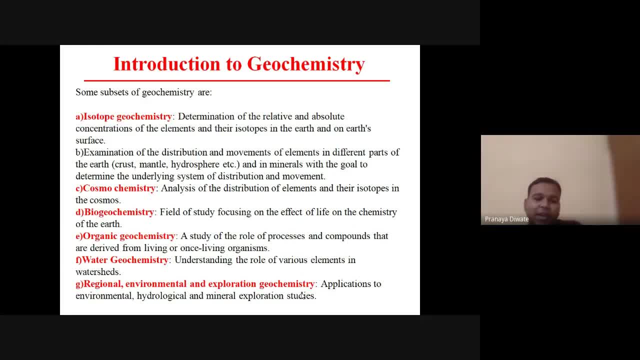 that is one, your biogeochemistry, then you have organic geochemistry, then you have organic geochemistry. so the organic geochemistry is a study of role of processes. organic geochemistry is a study of role of processes and compound готов gearide from the living or once. 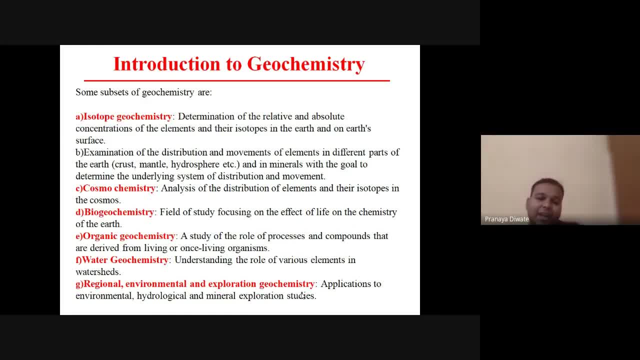 lean organism. so, whatever the organically derived sediment, organically derived drop, organically derived any component which we study under this, under the is branch, is known as the organic geochemistry, which is known as the organic geochemistry, then you have a water geochemistry, water. you know that all. what is the water? drinking water, and 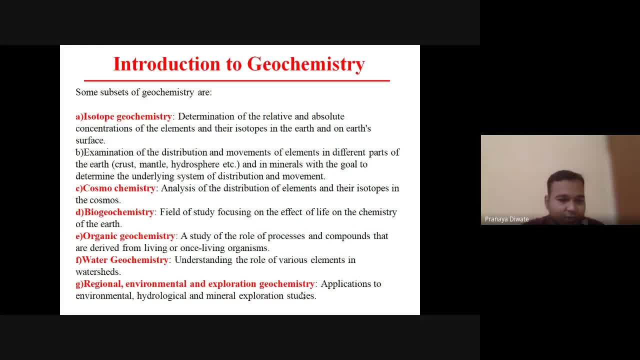 all this water, so that water- uh, geochemistry is when we study this lake and all the river water and all the element of this. all that is comes under the water geochemistry. okay, so understanding the role of various element in the watershed is comes under the water geochemistry. then you have 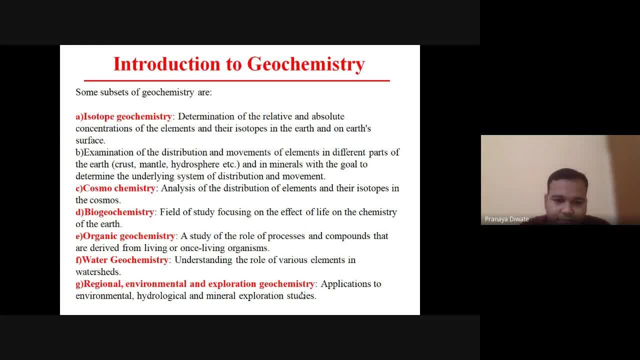 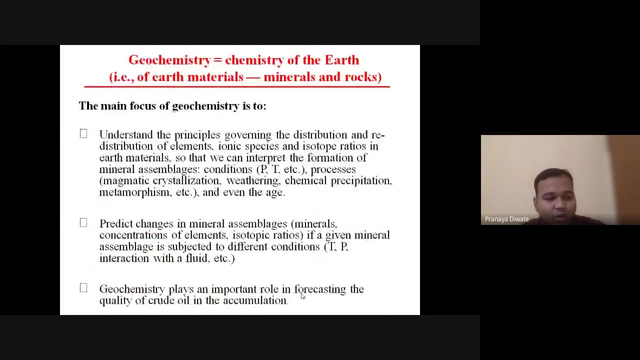 a regional, environmental and exploration geochemistry, then you have a regional, environmental and exploration geochemistry. so application to environment, hydrological, and application of environment, hydrological and mineral exploration studies comes under the what the exploration studies is. or we can have our exploration geochemistry. okay, so the geochemistry is the chemistry of earth, geochemistry is the study of earth. 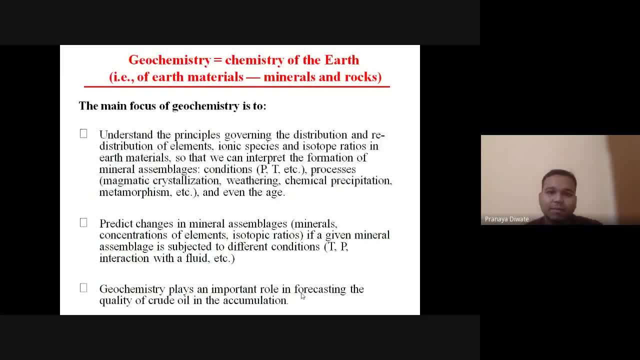 so, uh, earth has been studied. the earth material, geochemistry is the earth material and mineral of the rock. okay, so that is known as your geochemistry, that is known as your geochemistry. then you have what the main focus of geochemistry is. to what is the main focus of geochemistry? 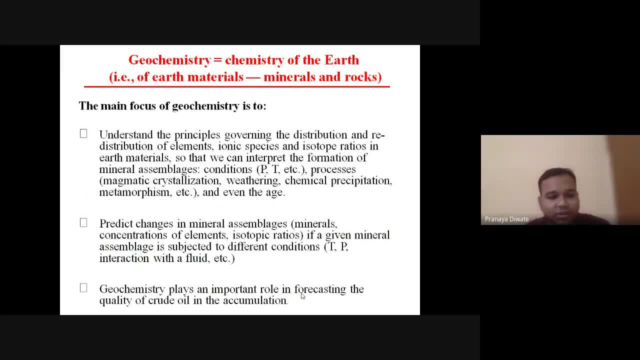 to understand the principle governing the distribution, understand the principle of distribution of the this one and redistribution of element, ionic, ionic species and isotope ratio in the earth material, in the earth material, so that so that we uh can interpret the formation of mineral assemblage, we can interpret the formation of mineral assemblage. 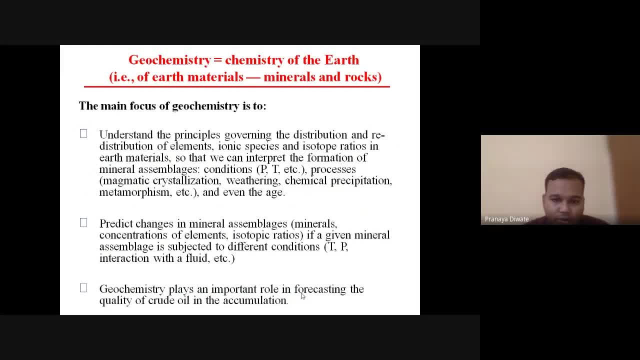 so uh. so what? what we are going to interpret? the formation of mineral assemblage, condition and processes, condition and processes. okay, so what? the processes? we have a magnetic uh, magnetic uh, magnetic, uh, constant crystallization, uh or uh, or we can have a chemical precipitation, metamorphism and even the age. so this is all. are the uh, all are the the main focus of the? 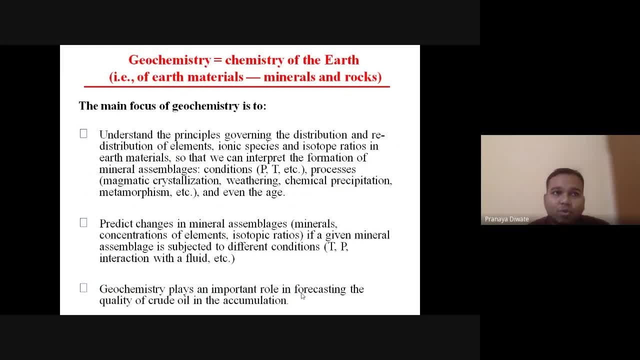 geochemistry. this is all. are the main focus of the geochemistry. what, then, other can do? the predict the. what we are going to predict the changes in the mineral assemblage. okay, we have to predict the changes in mineral assemblage if a given mineral assemblage is. 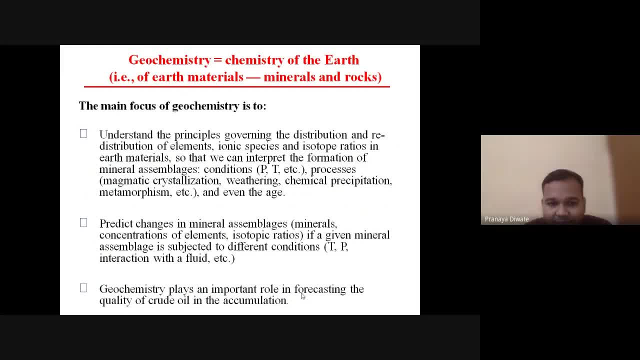 subjected to the different condition. if the, if a mineral, mineral assemblage is subjected to a different condition, that is, temperature, pressure, interaction with fluid and etc. they are also going to change the geochemistry. geochemistry هنا eş oldi an important role in forecasting the quality of crude oil in our accumulation. so the earth 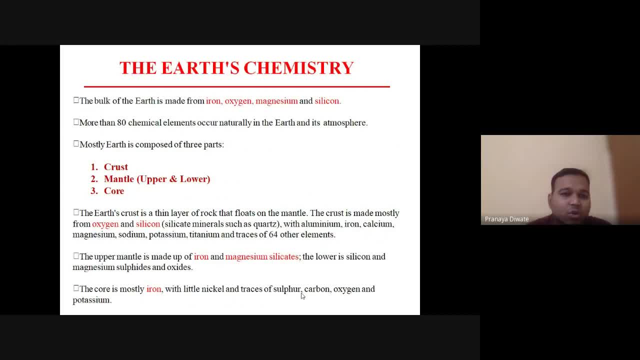 chemistry. so when we are going to talk about the earth chemistry. so earth- already we discussed that- divided into three different parts: crust, metal and core. earth is divided into three different parts: crust, metal and core. so the bulk of the earth made from the iron, oxygen, magnesium and 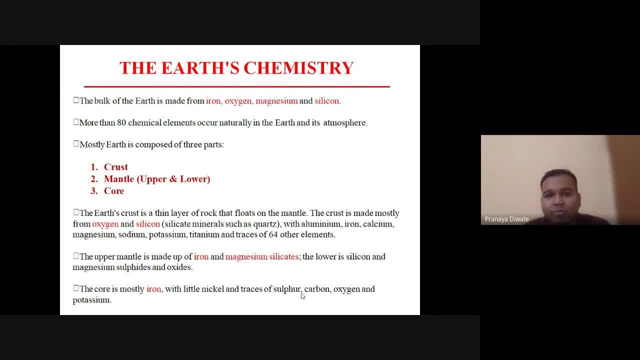 silicon. the bulk of the earth is made up from the iron, oxygen, magnesium and silicon. more than 80 chemical uh. more than 80 chemical elements occur naturally in the earth and its atmosphere. more than 80 chemical elements occur naturally in the earth and its atmosphere. mostly earth is composed of three part, that is, a crust, mental and core. 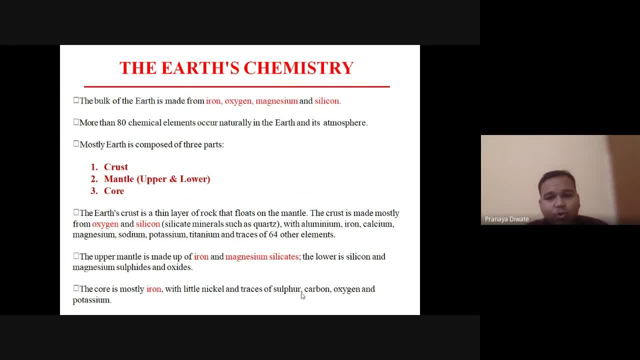 the earth crust is a thin layer of rock that float on the mantle. the earth crust is a thin layer of rock which is float on the mantle. the crust is made mostly from the oxygen and silicon. the crust is made from the thin layer of rock and metal. the crust is made mostly from the oxygen and 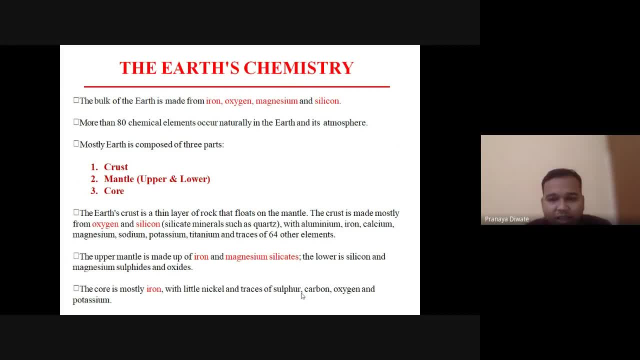 silicon crust is made mostly from the oxygen and silicon, with aluminum, iron, calcium, magnesium, sodium, titanium, titanium and traces of 64 other elements. so that is how the your crust is made up of то. the upper mental is made up of? uh, the upper mantle is made up of iron and magnesium silicate. 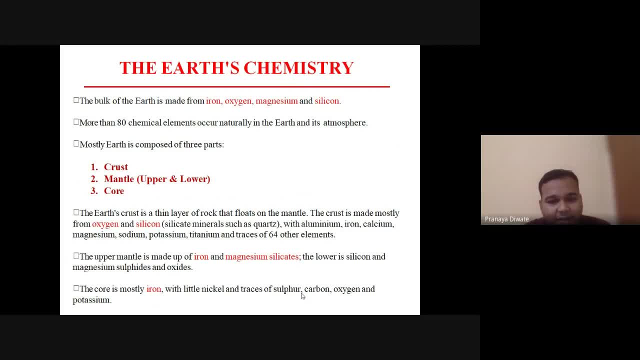 is made up of uh. the upper mantle is made of iron and magnesium silicate, the lower is a silicon and magnesium sulfide oxide. the core is mostly iron, with the little nickel and traces of sulfur, carbon and oxygen and potassium. so this is what about the earth crust and 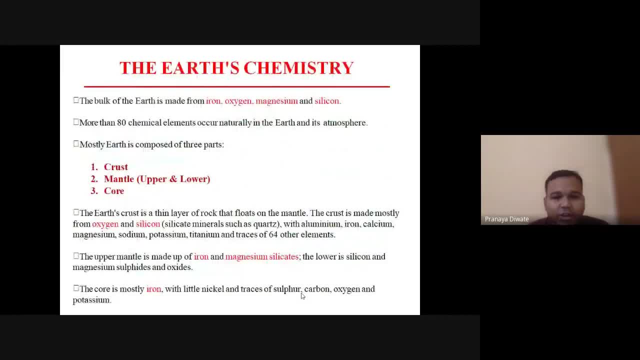 and earth crust and metal and down. you see mentor and core. so your crust is basically having a oxygen and silicone in their composition, or silicon in your. what composition of this one? then you have a mantle is made up from the iron and magnesium. the mantle is made up from the iron and magnesium silicate. the lower is the 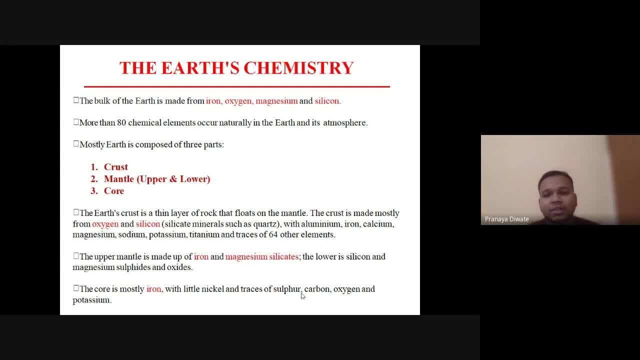 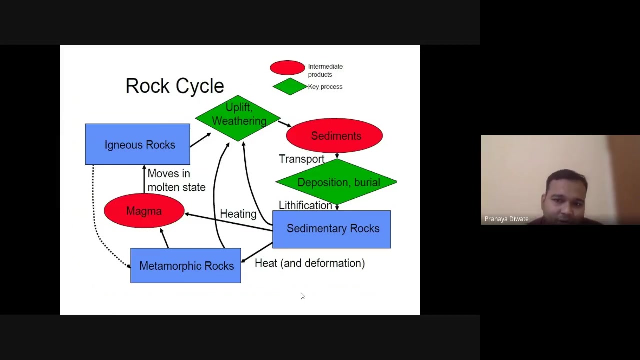 silicon and magnesium, sulfide and oxides. the lower is the silicon and magnesium and sulfide and oxide. the core is mostly iron. core is mostly iron with little nickel and traces of sulfur, carbon oxygen and potassium. so this is all about the crust mentor and core. so the rock cycle is all about the. what is the rock cycle, how it is going on. igneous rock, which 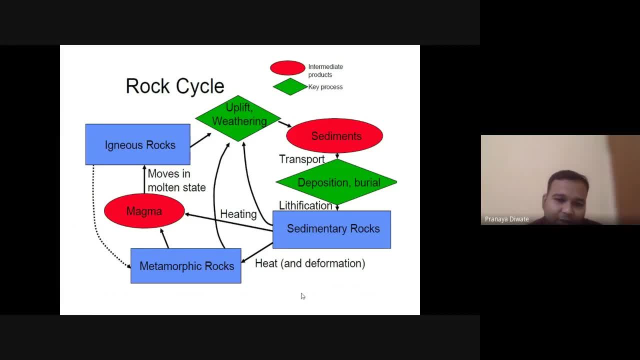 is converted to the sedimentary one and then it is converted to the metamorphic rock. but in between you have a processes. we already have one separate video on the rock cycle. you can refer that video, but here we can just take a one. uh, a brief about a very short introduction about how. 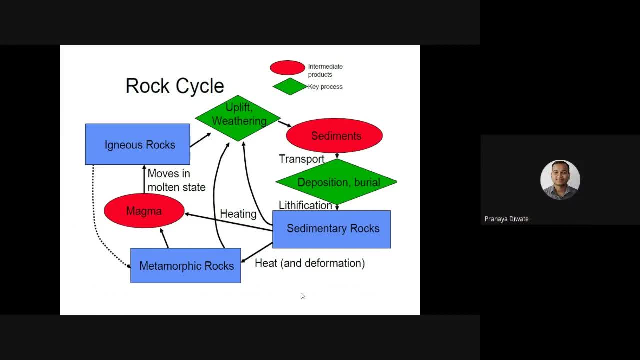 rock cycle is nothing but the uh, a cycling of the one one rock type to the another, another to one. so so you are, igneous rock is converted to the sedimentary rock, by which process, a flip man weathering, then you form a sediment, and sediment get deposited and burial and the lithified one, so that 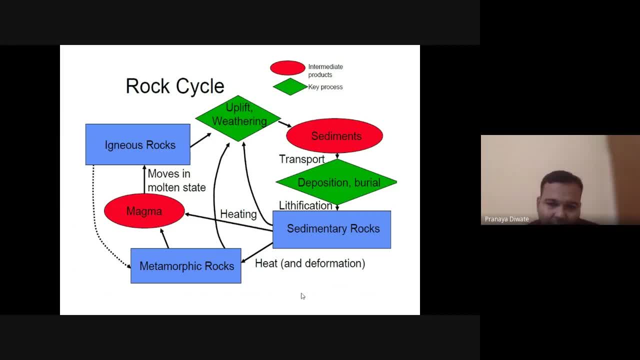 lithified rock is having a known as sedimentary rock. that lithified rock is known as sedimentary rock. then you have a metamorphic rock, then you have a metamorphic rock. so metamorphic rock is converted by the heat, converted by the heat and deformation. metamorphic rock is converted by the 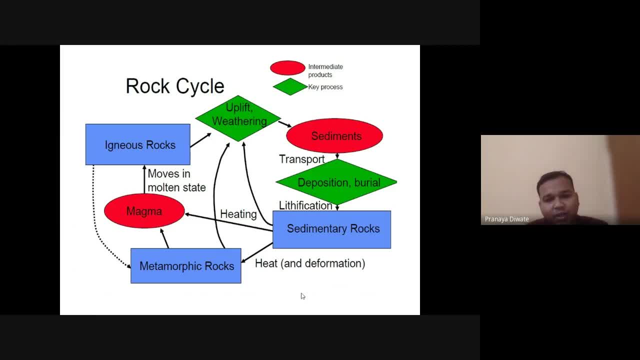 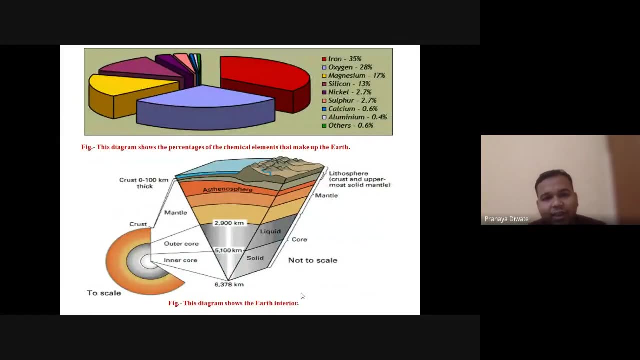 heat and deformation, the metamorphic rock can again get uh, having some heating and all this phenomena which converted the metabolic rock into magma, into the magma. so this is the diagram which shows the percentage of chemical element. this is the diagram which shows the percentage of chemical element. 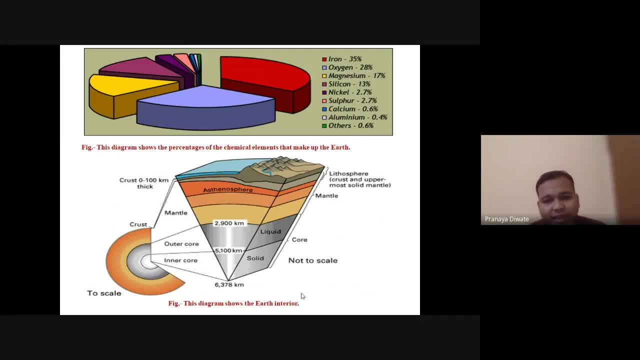 which makes up the rock. this is a diagram which shows the percentage of the chemical element that make up the earth, which will make up the earth. so you have a lithosphere. okay, so? so this is the how the earth is all about. what is the composition of? if anybody asks you what is the composition of earth, you can have this diagram. 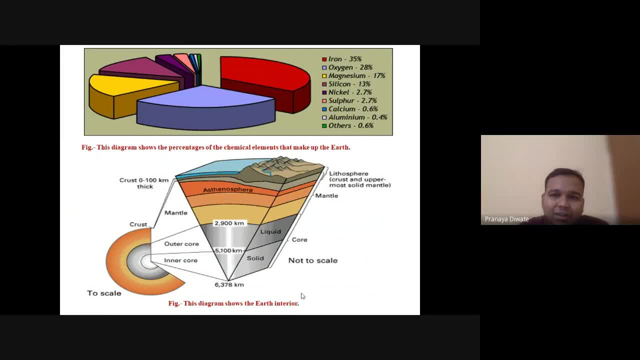 this is the pie chart of the means type of pie chart. so you have iron, you have oxygen, magnesium, silicon, nickel, sulfur, calcium, aluminium and other. so this is a element which is having a more than 0.5 percentage of the concentration in the oil. how the iron is having so much of percentage? because 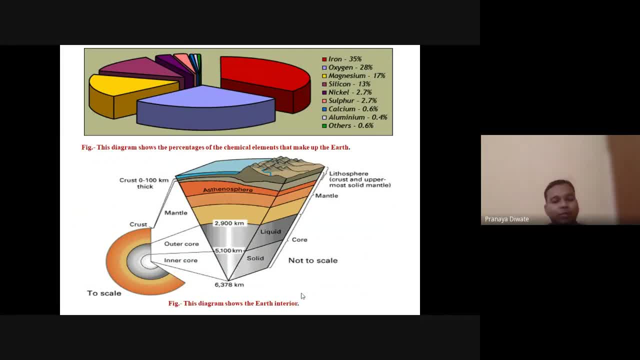 in a core, basically in an inner core, you have mostly, you have mostly uh. you have mostly iron in your uh core. you have a iron in your hole, so that's how you have a uh, iron, oxygen, magnesium and that's one. so then you have uh, uh, your earth, which is uh we already discussed about. 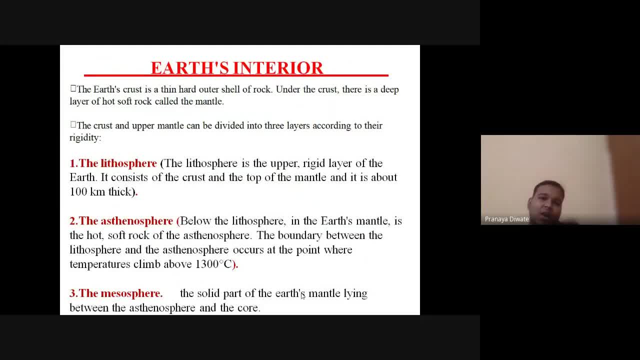 so all crust is a thin, hard, uh, outer shell of the rock. under the crust there is a deep layer of the hot, soft rock called the mantle. so earth is earth. crust is a thin, hard outer shell of the rock. the earth crust is a thin, hard outer shell of the rock. 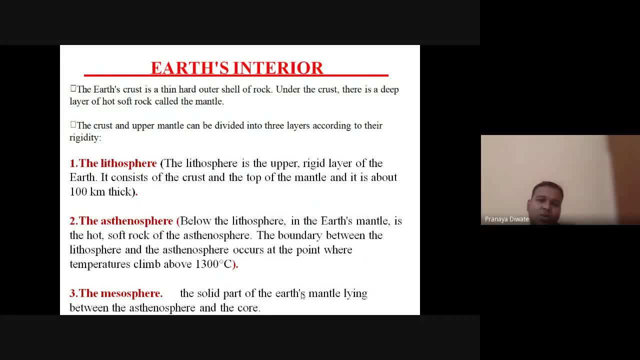 which, under the crust, there is a deep layer of the hot soft rock called the mantle. the crust and the upper mantle can be divided into three layer according to their rigidity. the crust and metal. uh can be divided into three layer according to their rigidity. uh can be divided into three layer according to their rigidity. the lithosphere- the lithosphere is the 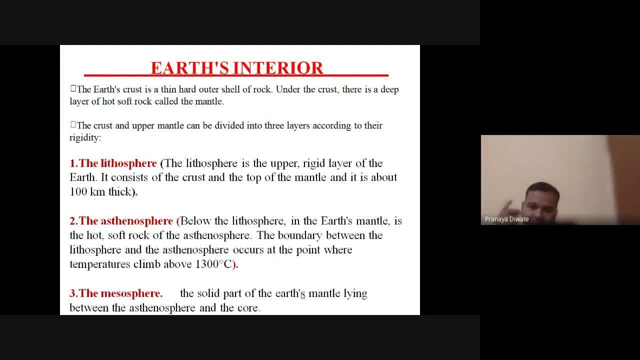 upper rigid layer of the earth. the lithosphere is the upper rigid layer of the earth. it consists of the crust and the top of the mantle and it is about the hundred kilometer thick. it is about a hundred kilometer thick. second one is the astonosphere. the astonosphere is below the 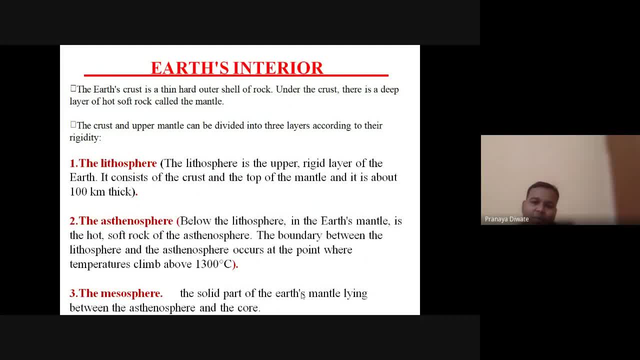 lithosphere is the earth mantle, which is hot, soft rock of the astonosphere. the boundary between the lithosphere and the astronomosphere occur at a point where temperature click above the 1300 degree celsius. so this is a uh astonosphere. so lithosphere is there, astonosphere is there and 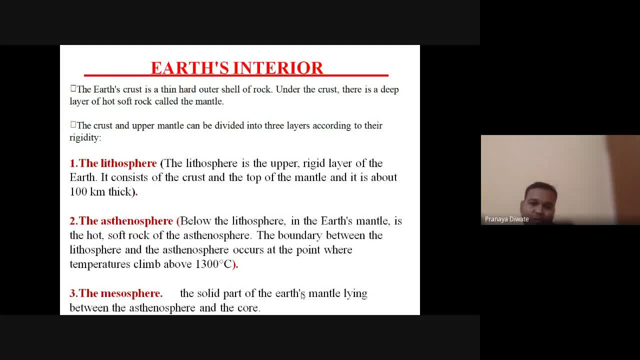 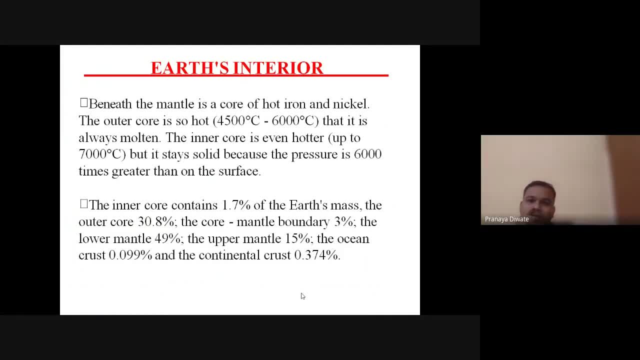 the mesosphere is there. so you have a astronosphere, lithosphere and lithosphere and mesosphere. this is the three different layer of the ores beneath the mantle. uh, beneath the mantle there is a core of. the outer core is so hot that it is always molten. the inner core is always even hotter, up to 7000. 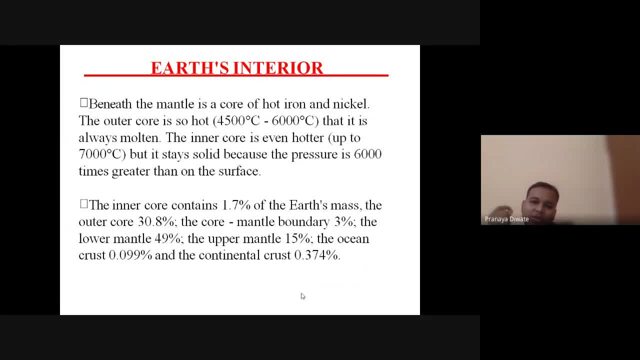 degree celsius, but it stays solid because the pressure is 6000 degree celsius, 6000 times better than on the surface. so the inner core contain 1.7 of the earth mass, the outer core is 13.0 and 13.8 of the core. mental boundary is three percent. the lower mental is 49 percent. 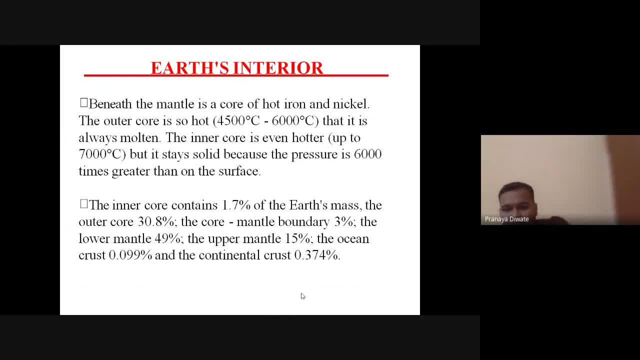 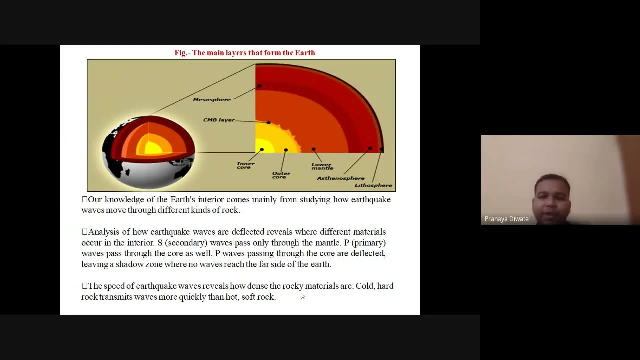 this is how you can have a different percentage of the your iron and nickel. iron and nickel. so to our knowledge, to our knowledge, the earth interior comes mainly from the studying how the earthquake waves moves through the different kind of crops. so knowledge of the earth's interiors only comes from the, mainly from the studying how earthquake existem. 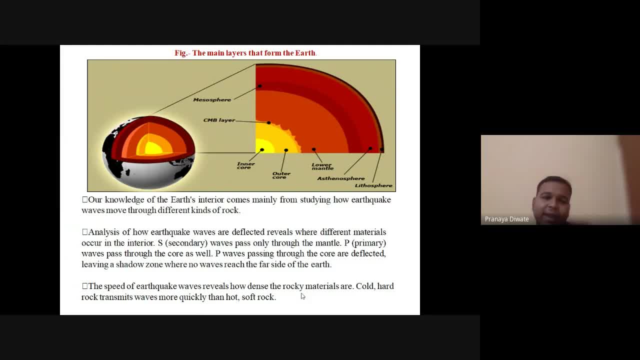 waves moves through the different kind of law, and this is how earthquake views are deflected, reveal where the different material offer in the interior- yes, is the avails, which is passed laterally through the mental bills pass through the or as well. T was passing through the. 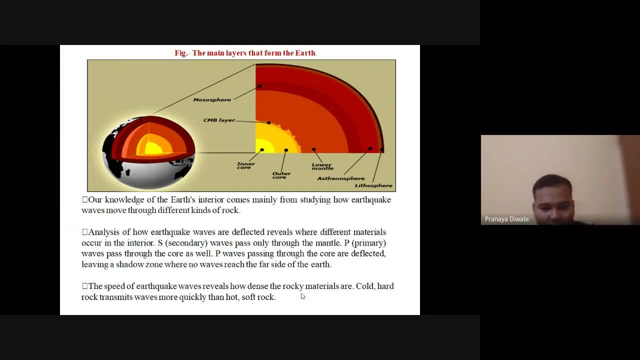 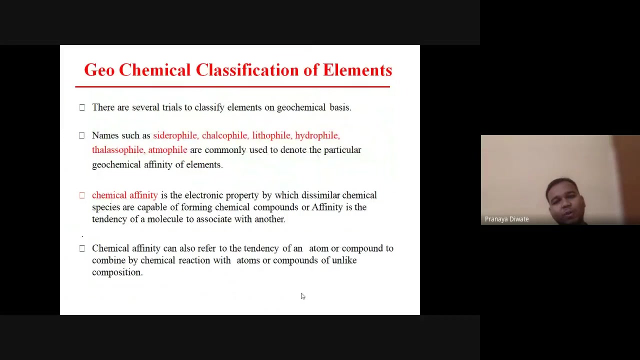 under the and deflected a living a shadow zone. which is giving a shadow zone or the speed of the earthquake will reveal how days rocky material are. old hard rock pass me there was more quickly than the soft and hard rock. the geochemical classification of element. geochemical classification of element. there are. 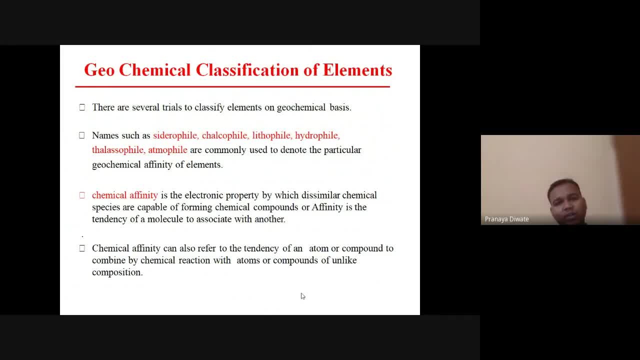 several trials. there are several trials to classify element on geochemical basis. names such as Cedro, Cedro file, chalco file with opine, hydroponel, elastopine, at most at mo file, which are the commonly used to donate. you know the particular geochemical operative element. what is the chemical affinity, the 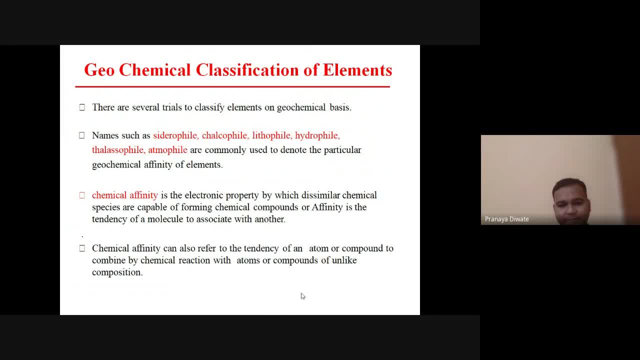 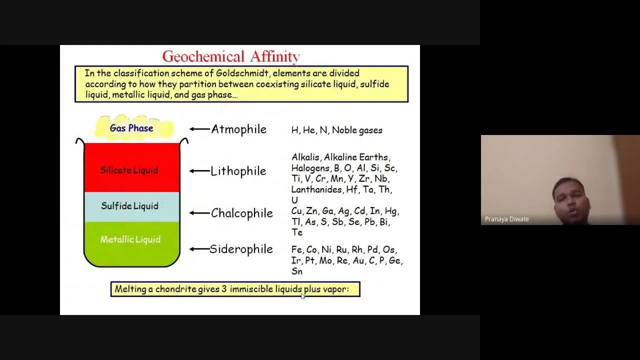 chemical affinity is the chemical affinity between the elements of the electronic property by which dissimilar chemical species are. so this is what your classification of element is based upon. so what is the geochemical affinity in the classification scheme, the goldsmith, who is the one of the 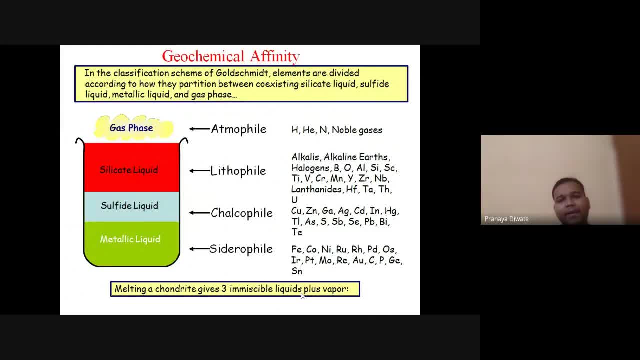 greatest scientists for the chemistry and all which divide the element, according to their how they are passion, how their partition between the coexisted silicate liquid suffice liquid as metallic liquid and gas case. so you have a atma file Ethel by chalco violence hydro pipe. this is a port. 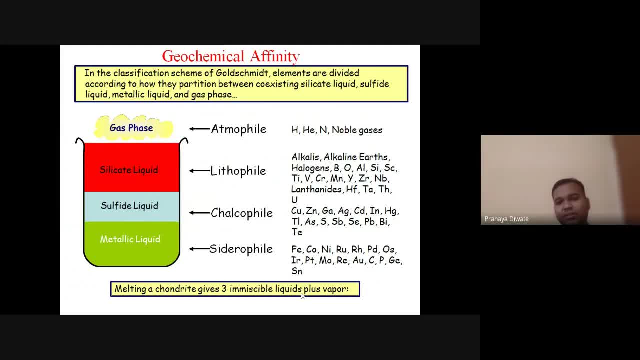 different kind of component. which? which geochemical opinion is that so? so you have a silicate with, obviously, you have a, or silica alumina, and this all are the known as the lithophile. all the gas phase element is known as the, all the gas is all known as the hydrogen, and you have a surface liquid. then you have a. 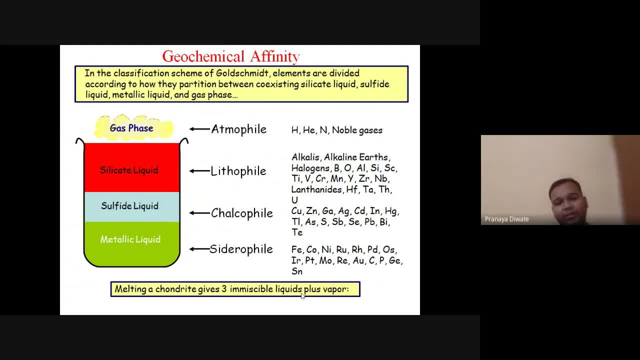 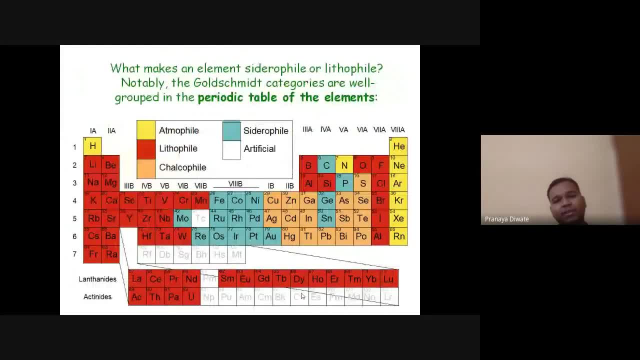 surface liquid. that is a chalco file and see profile. then you have a water makes the elements you profile or little file, not notably that goldsmith, categorize our well group in the period table of the element. so the atmo file, citroen file. 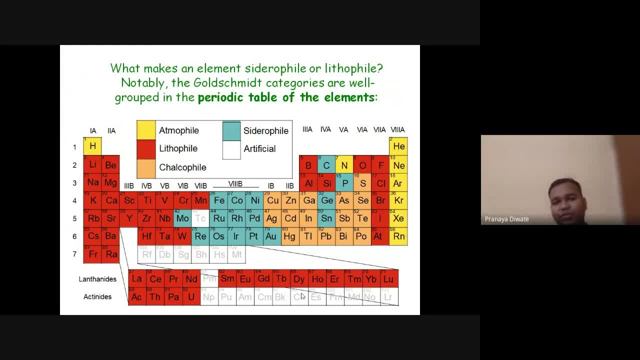 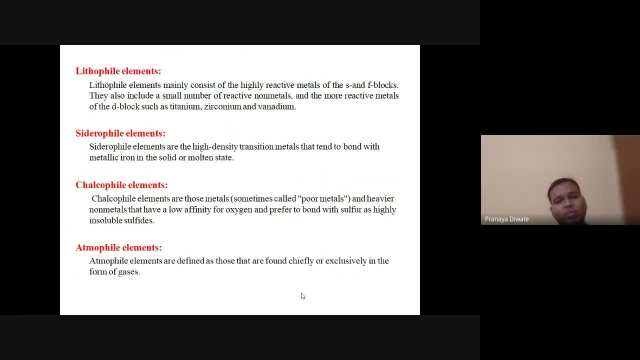 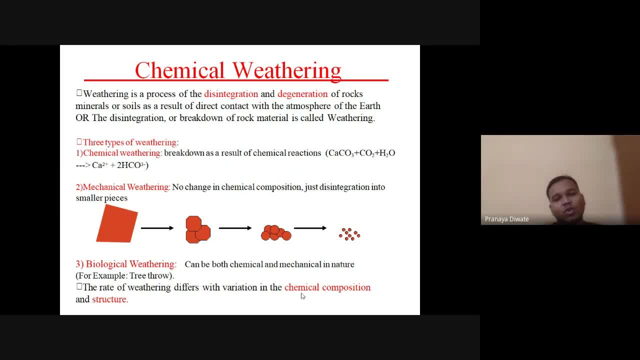 bit of a liquid. so this is a little bit of a liquid. so this is a little bit of a liquid. regeneration of rock, middle or the soil as a result of direct contact with the atmosphere of the earth or the distinct or breakdown of the earth material is. 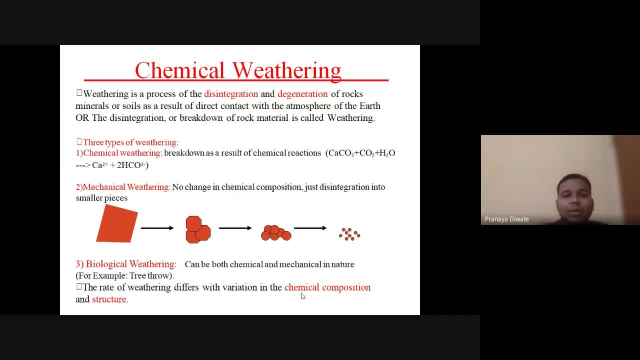 called the weathering. so there is a three type of weathering, are there? there is a three type of weathering. are there a chemical weathering, mechanical weathering and biological weathering. so while in the chemical weathering there is a breakdown of a result of chemical reaction, then you have mechanical. 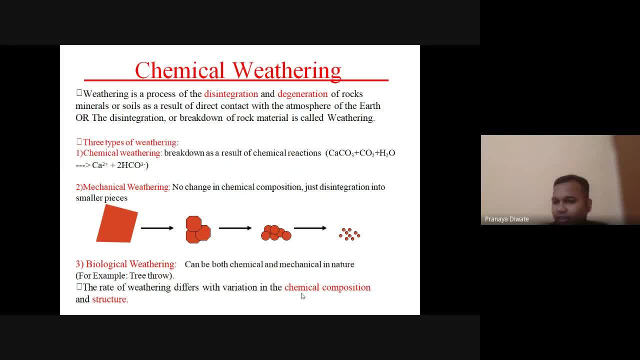 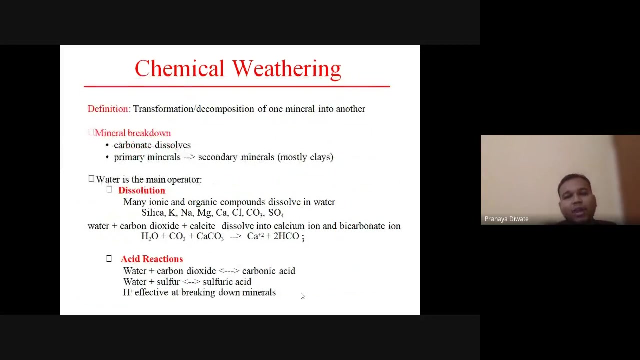 weathering. no change in a chemical composition, just disintegration into the smaller pieces. then you have a biological weathering. biological weathering. biological weathering can be both chemical and mechanical in nature, so you have a different type of chemical weathering in. then you have mineral breakdown. the mineral breakdown is breakdown. the carbonate dissolve and 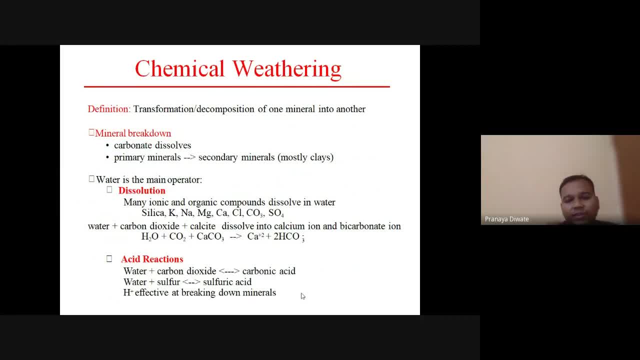 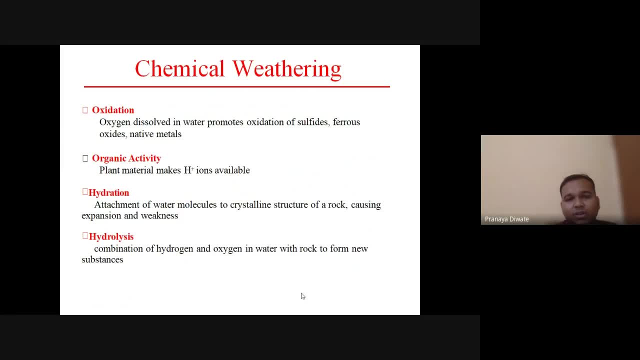 all water is the main operator for this. all the weathering, also the acid when you have oxygen, when you have addition of oxygen to promote oxidation and oxidation and organic activity. so this all are your, what we can see the operation of the chemical with me. then you have a hydration and hydrolysis, then you have a 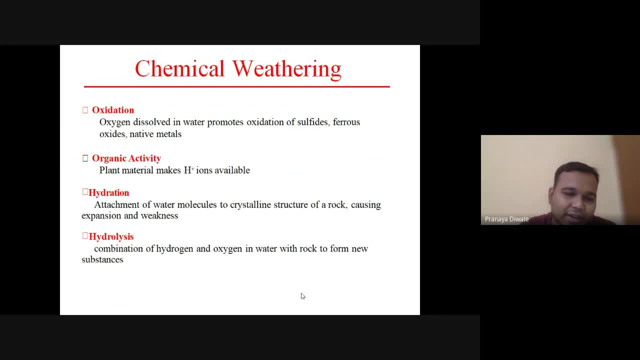 hydration and hydrolysis. what is the height? what is the hydrolysis? our hydration is a attachment of water molecule to the crystallized structure of rock, causing expansion and weathering, whereas the combination of hydrogen and oxygen in water with the rock to form on new. 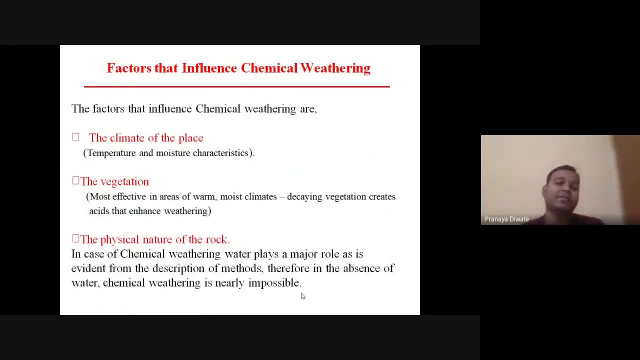 substances, the factor which is infrared, the chemical weathering. what is the factor which is the chemical weathering? the climate of the place. so, whatever the climate of the particular place, whether it is a unique weather, is the cold weather in the hot. so you have a different kind of climate and the the 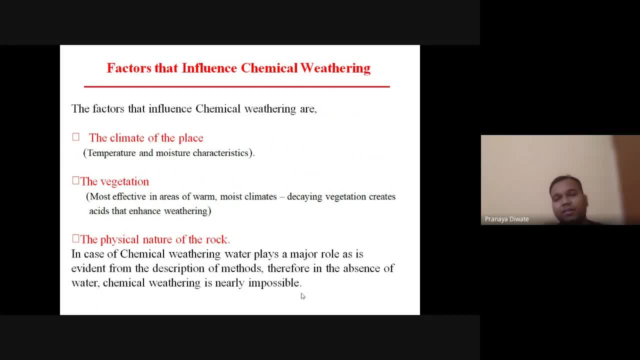 different type of climate is having a different kind of effect, a different kind of planning. planning you have a different kind of. if it then the vegetation, the most you can do, the most effective in areas of warm, moist climate, decaying the vegetation creator, this one, so the physical nature of them all, so all of 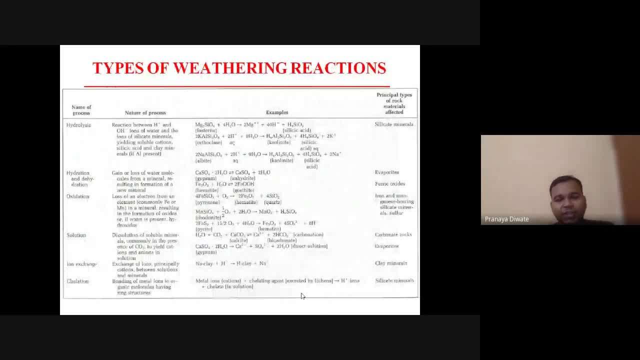 these are the influencing the chemical weathering. there is a different type of capable within. we already seen a hydrolysis. I addition stops: hydrogen oxygen, calcium, penisiane, hydrogen calcium, potassium and iron destination, so iron of exchange. so these all are the wedding analysis. then you have a geochemical analysis. 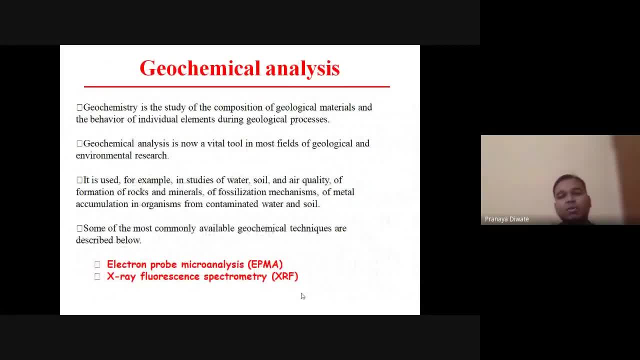 then you have a geochemical analysis. so geochemistry is the study of composition, geochemistry is the study of the component of geological material and the behavior of the individual element during the geological process. a geochemical uh, geochemical uh analysis is now to vital, now to a vital role in a tool in the most field of 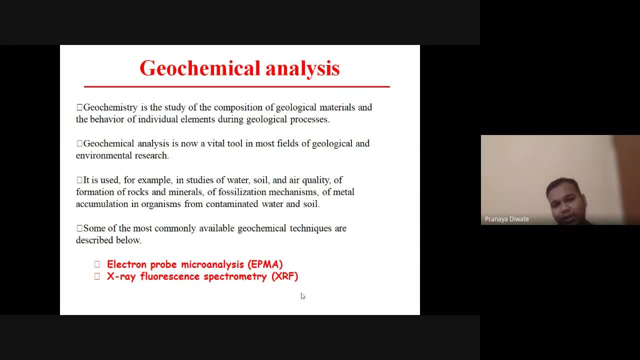 geochemical, geological and fundamental research. it is used, for the example, in studies of water, soil and air quality, of formation of rock and mineral, of fossilization mechanism, some of the most recently so uh. geochemistry is the study of the composition of geological material, which is behavior of 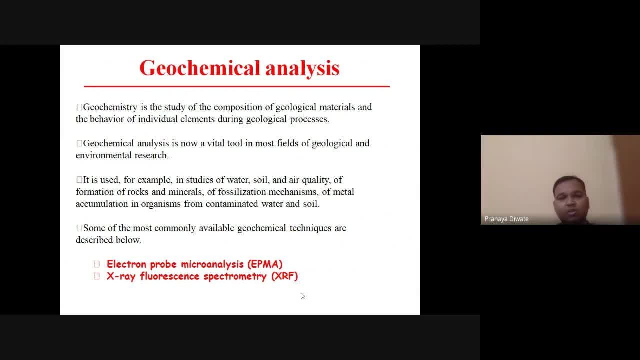 individual element and, uh the what? when we are going to see how we are going to use the different kind of analysis. so you are going to see the geochemical analysis, which is the most important part for the geochemistry, geochemical analysis. geochemistry is the study of composition, geological. 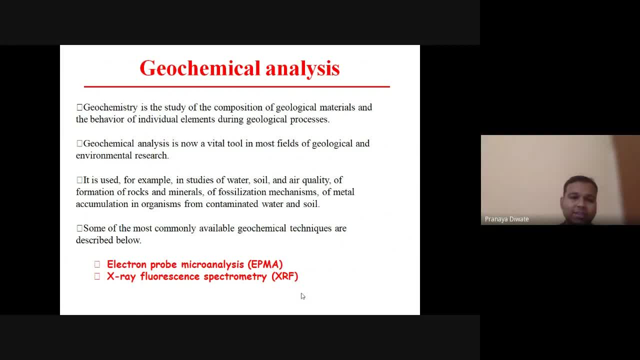 material. so in geochemistry, the study of composition of rock material, and so geochemical analysis, is now the vital tool to most field of geological and natural research. it is used, for example, in studies of water, soil and air quality, of the formation of rock and mineral. so so the it is having a analyzed by the different kind of instrument. 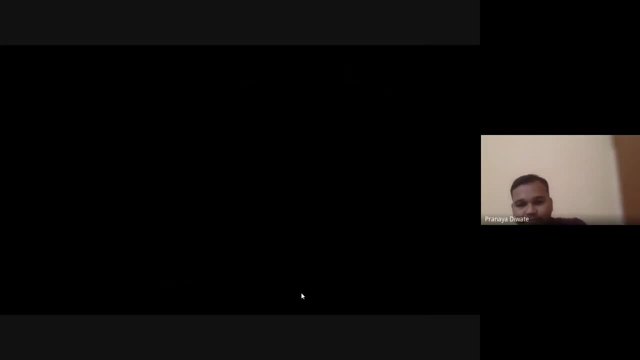 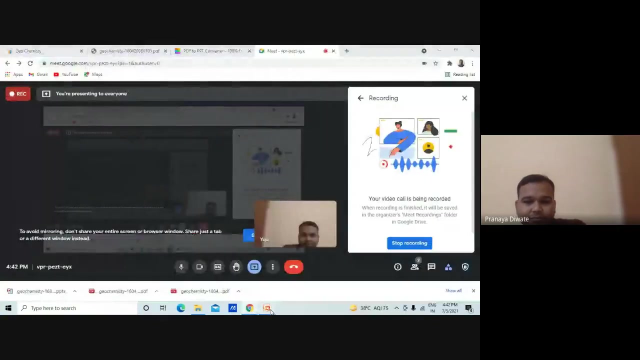 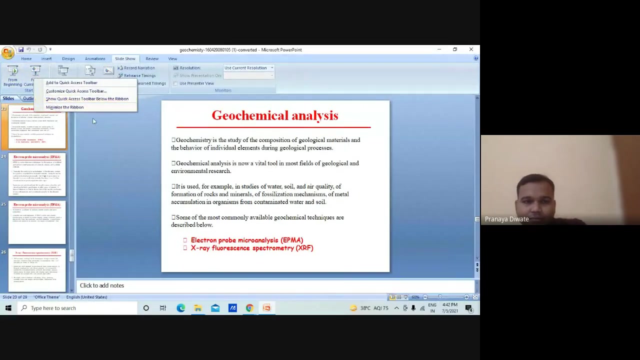 so we have here apm and x-ray fluorescence. epi and x-ray pollution is the only remaining here. so you have an electron probe, micro analysis, e, pma. so you have a macró analysis is epma and you have a x-ray fluorescence. so what these are, we are going to see. 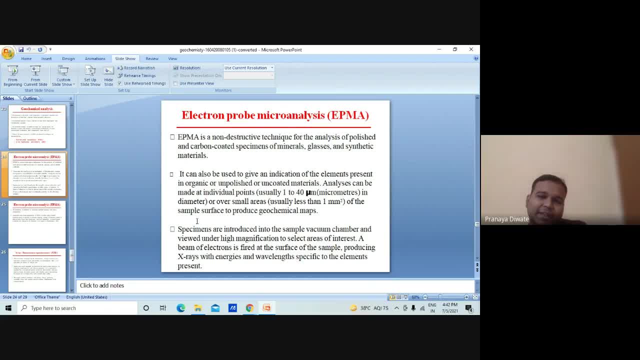 so what is the epma? epno is basically a instrument. epma is a basically an instrument which is non-destructive, which is a non-destructive technique for the analysis of polish and carbon coated specimen of mineral glasses and synthetic mineral. it can also be used to give the uh indication of element prepared, uh, inorganic or unpublished. unquote. 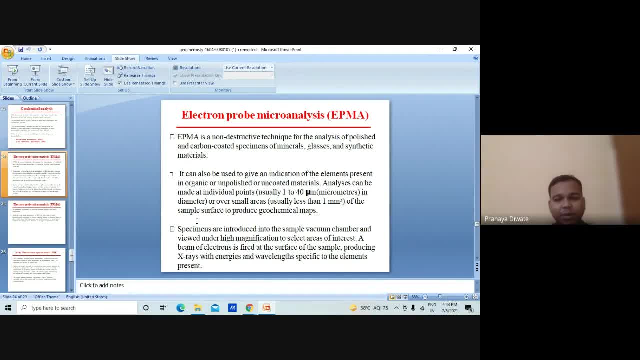 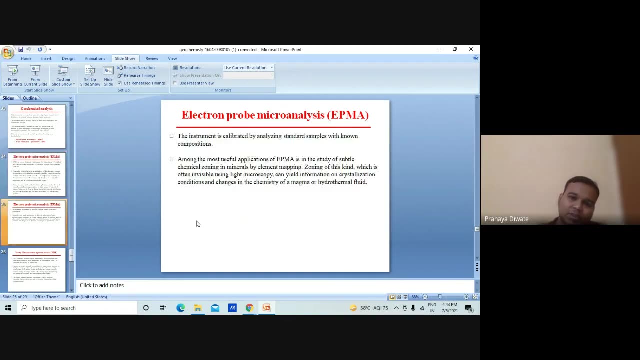 so these all are the uh epma about. so the specimen, uh specimens, are introduced into the sample vacuum chamber and these all are the known as the epma technique. so this instrument is calibrated, analyzing standard with known composition among the most useful uh, composition among the most uh. 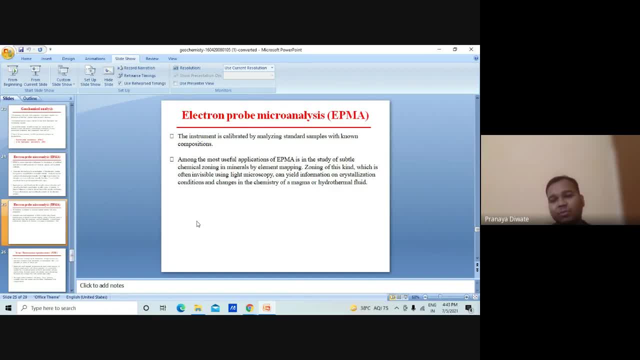 so the most useful appreciation of epma is the study of sub subtle uh chemical zoning in the this one. so uh zoning of this kind, which is often invisible zoning, is required for the this one. so the most useful appreciation of epma is the study of sub subtle uh chemical zoning in the 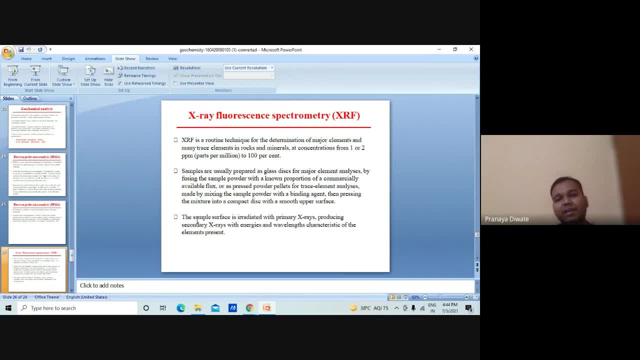 very basic of the body is the study of sub subtle uh chemical zoning in the then. second one is a x-ray fluorescence spectroscopy. that is also known as xrf. many people are doing this for the mineral composition also. and uh, this, uh, what we can say, the a different kind of uh analysis, what we are. 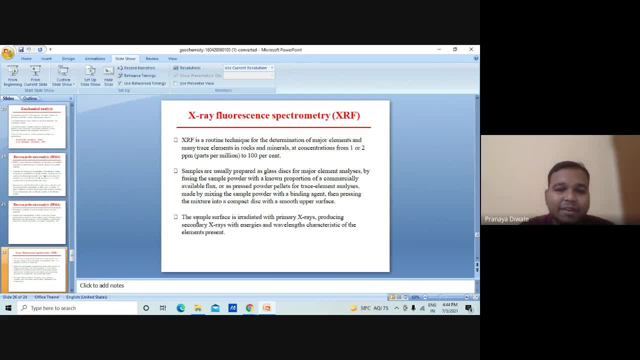 going to see. so xrf, that is, the x-ray fluorescence. xrf is a. x-ray fluorescence is a routine technique element in the drop, its concentration from the. its concentration is from the, what we can say, the. so, uh, the sample are usually prepared as a glass disk and major element, a major element. 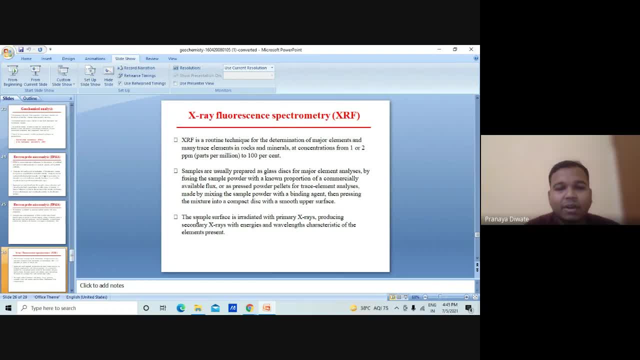 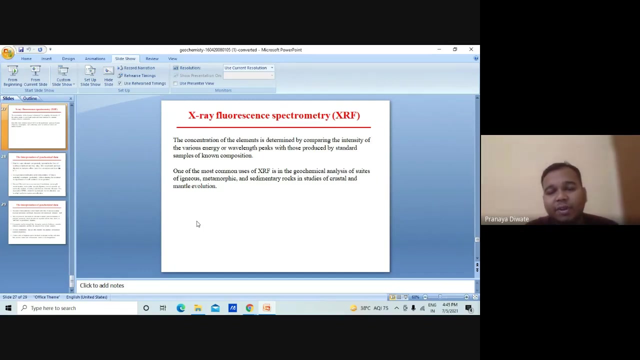 analysis by fusing the sample power and with the known parameter of commercially uh available flux. so other other other press powder, powder and this, all this all are get through primary x-ray. so this is what a mechanism of x-ray: the concentration of element is determined, the comparing the intensity of various uh. 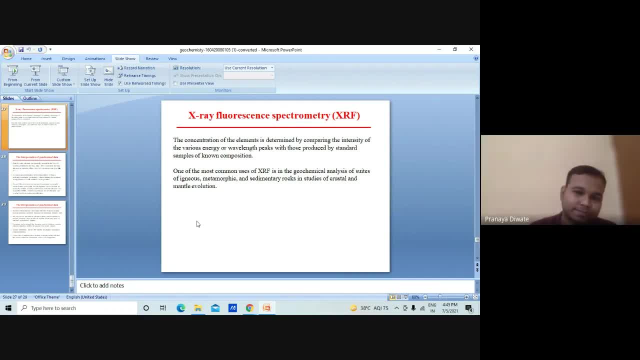 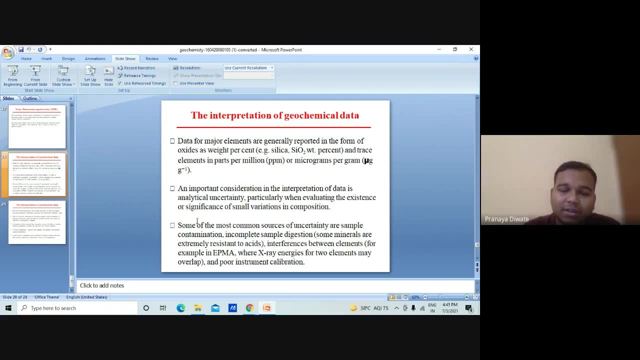 depression you so the interpretation of geochemical data, how you are going to interpret the geochemical data. the data for major element are generally uh. so the the important of considering those uh analysis, uncertainty, practical all are the important one. some of the most common source of the uncertainty are the sample. 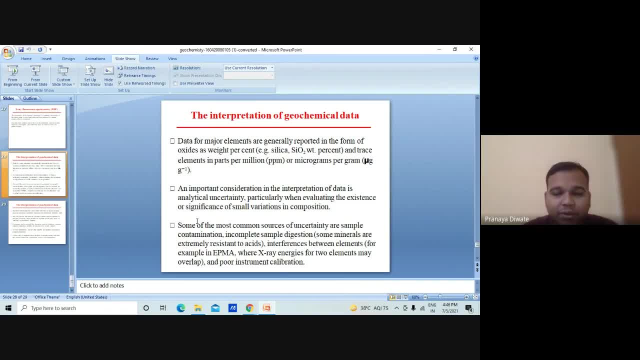 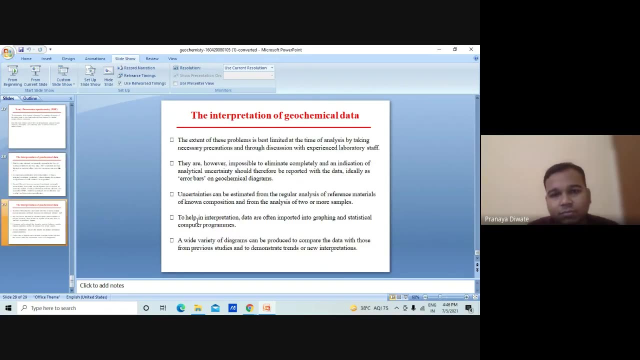 uh sample contamination: incomplete sample uh. so so you have a interpretation of this geochemical data which is derived from your xrf and xrd study in all. so the extent of this problem is being limited to the time of analysis by taking uh uh or taking up what we can say. 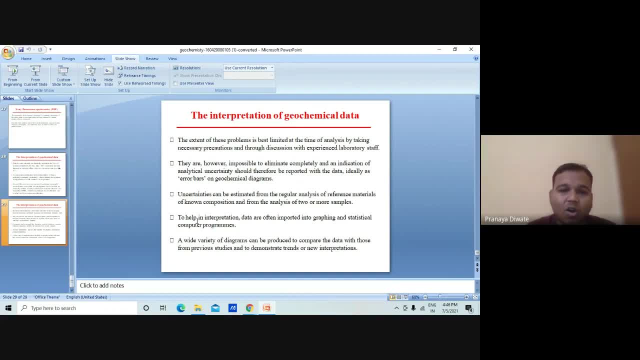 what we are going to see? uh, they are, uh, however, impossible to eliminate completely, and indication of analytical uncertainty should therefore be reported with the data. so, uh, so the uncertainty can be estimated. uncertainty can be estimated from the regular analysis of references, from the regular analysis of references. 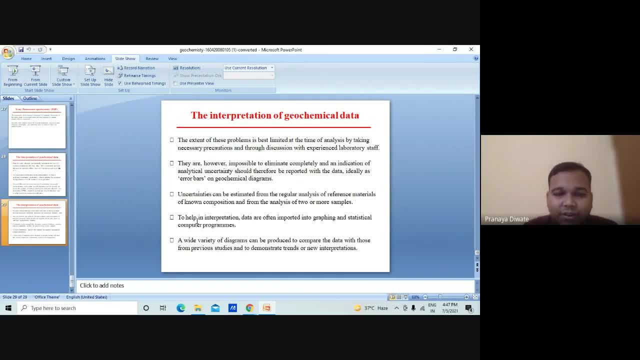 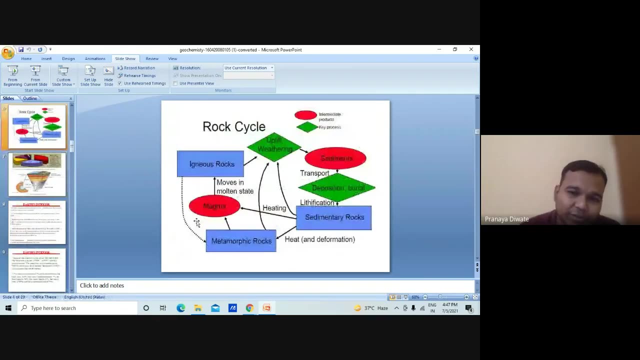 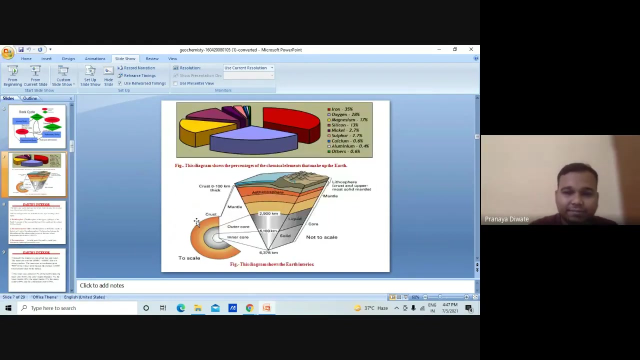 of reference. i can open it up. so i'm going to clear it up here. Niagara. uh, however, you see different탄. Yeah, am i hitting the solution? you can see it doesn't falling away from the initial solution. um so, um, all d larger. So. 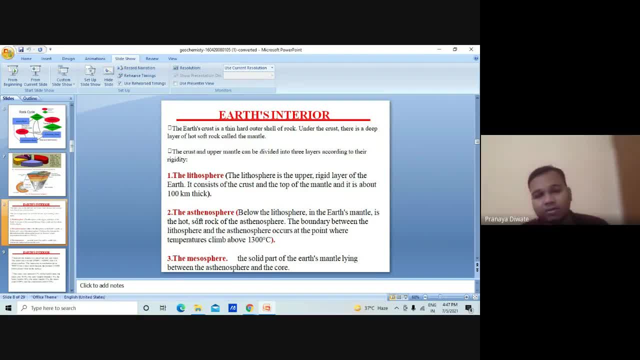 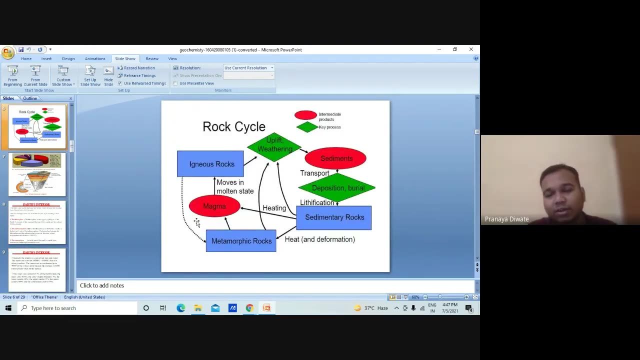 uh, the temperature've been more practical. We are going to study, maybe, This one. so the art is divided into the three different parts, with those clear, Astros clear and the mythos clear. This is clear. So the sediment which is going to the deposit, and burial sediment which is deposited and barrier into the 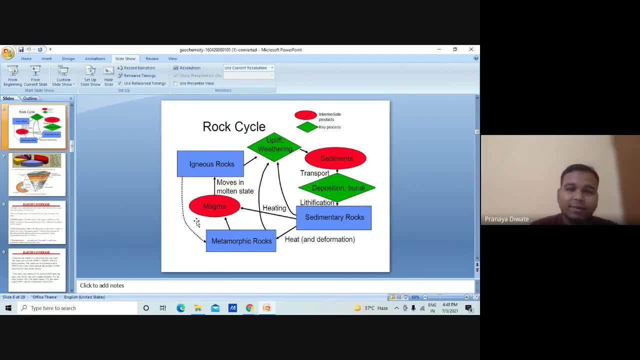 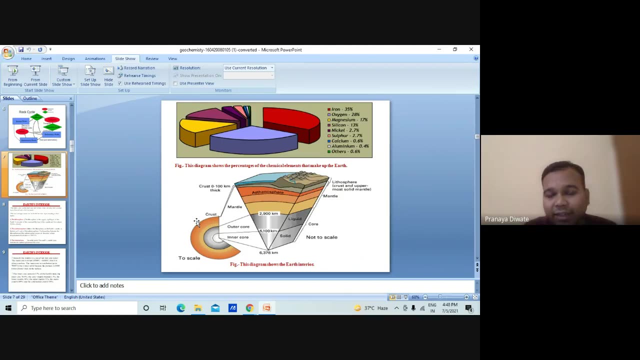 This rock cycle, So rock cycle, is nothing but a cyclicity of though. Oh, with one rocket converted to the another, another get converted to the one. This is what your rock cycle is there. Then you have more highest. What the gravitational pull is taking up from in the earth surface, That is all- are the mostly the granite. 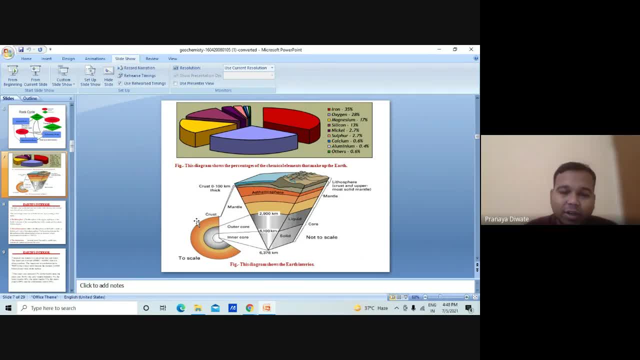 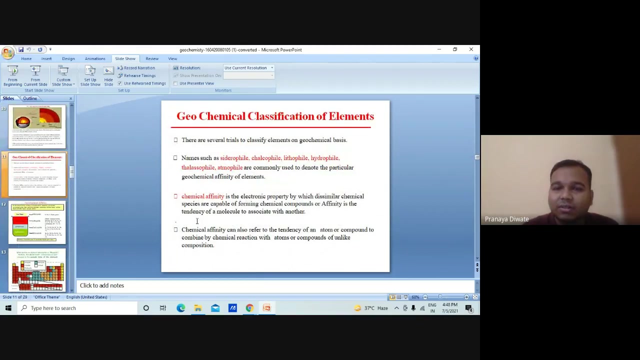 granite is So granite. so you are. what percentage of the chemical elements? percentage of the chemical element iron and oxygen. so iron is Basically forming a core and that contribute up many more. Then you know all. we already seen the earth. then we have a geochemical In a geochemical. 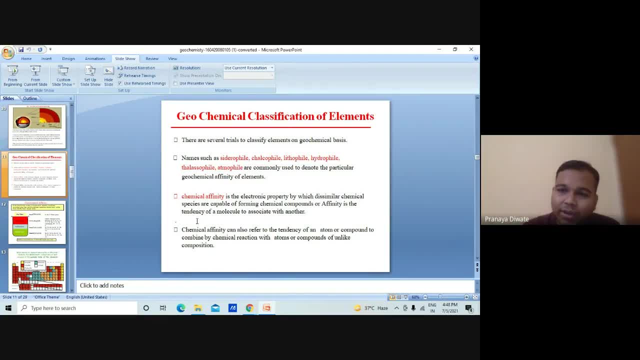 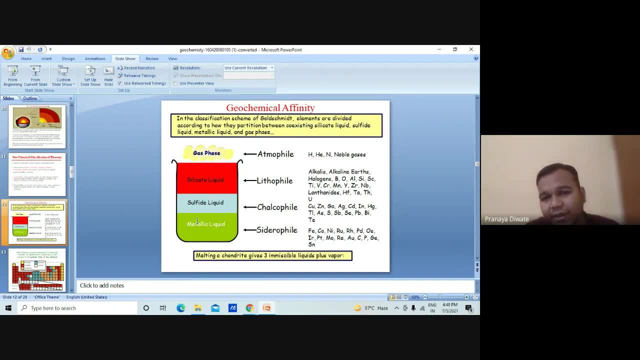 Chemical, with the geochemical, chemical classification of the element Are. also we seen the geochemical affinity which, which mineral, which element get up here? Take one Element from the other. so to avoid this one, We are just Having a Google. So so the this is the geochemical affinity of the 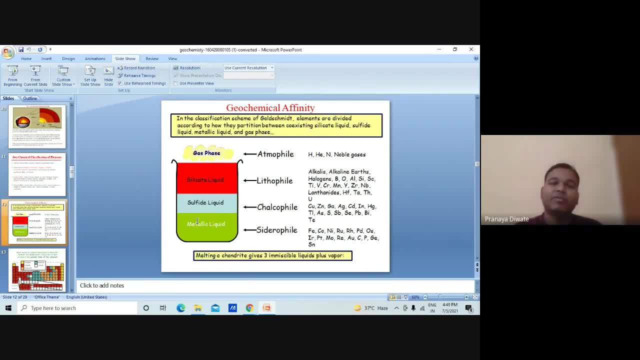 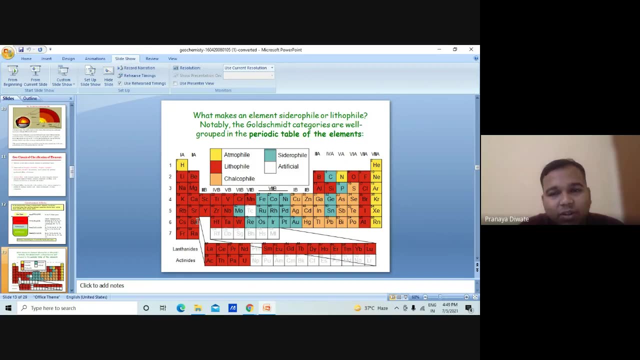 material. This is a geochemical affinity of the any What we can say, them any Things you cannot be. So what makes the elements? Hydrophilic opal, notably the goldsmith, is categorized? well, nobody, nobody. the The goldsmith categorization are well ground to group in the periodic table of the 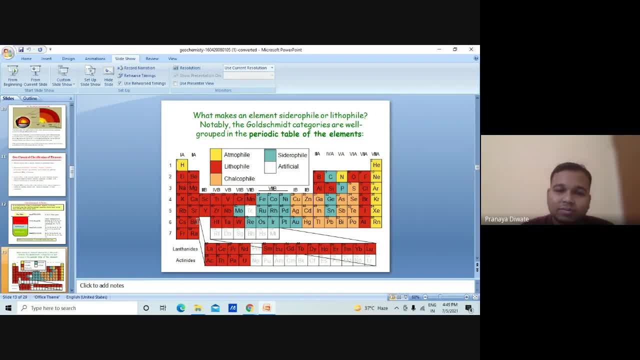 So you have and people it goes for little files and this all. so you have a this syndrome file and atmosphere and little file and Chalcochli I write. Chalcochle like this is all about the different kind of element We have. 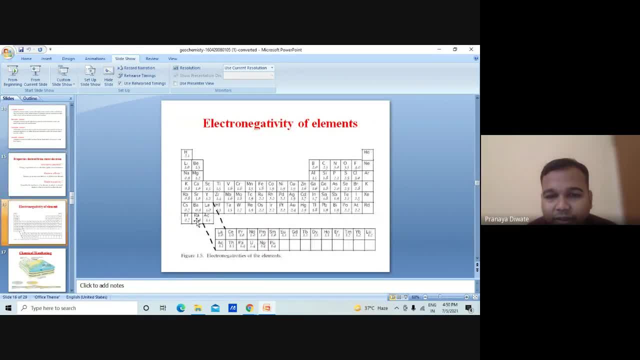 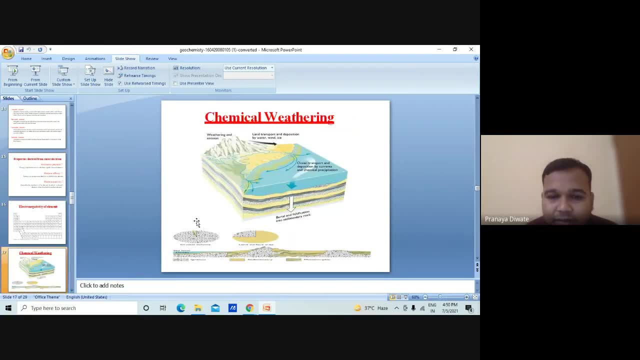 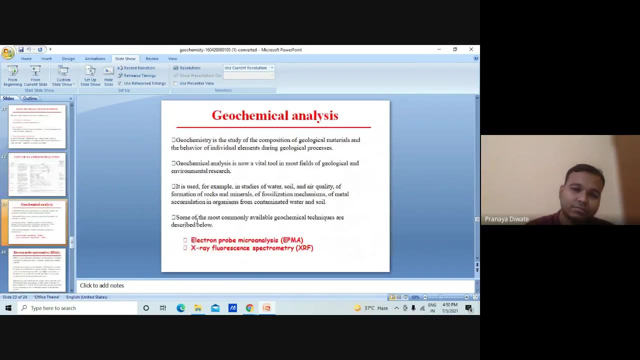 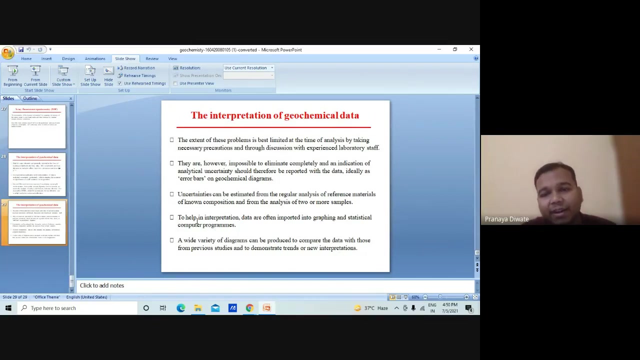 This is a property which is derived from the outer muscle. This is a temperature, This is a temperature, and So You uh extent of this problem is best limited at the time of analysis by taking the, by taking the, their, this one uh. so the to help the interpretation, data are often imported uh. 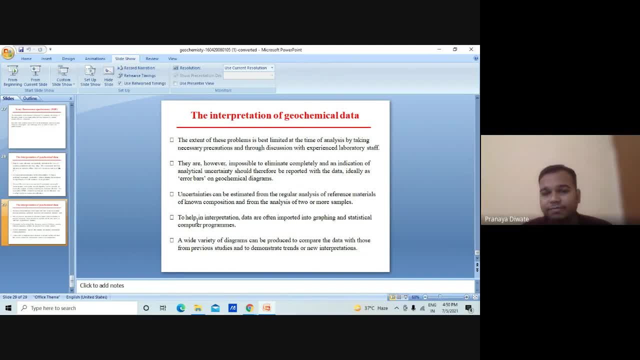 graphic and statistical. uh, a wide variety, a wide variety of the diagram can be. the diagram can be produced to compare the. so these all are the best example and a general introduction about the geochemistry. again, the geochemistry is a very large branch. you can, whenever and from whatever the place you are. 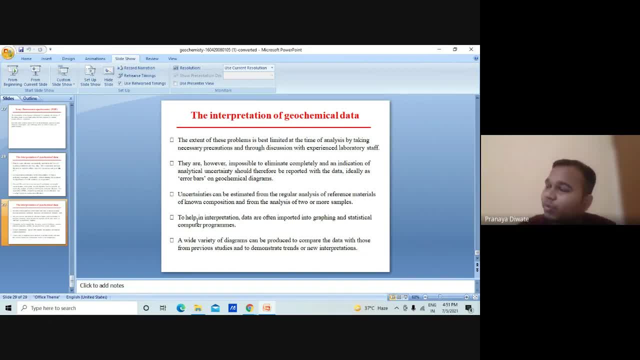 just taking the plot and this wall, you can also find it here. so the uh, so the interpretation of geochemical data is consists of the this one: okay, so uh, what is all about the interpretation of geochemical data? what about the international uh, uh, so uh, this all are the geochemistry. now, what is the application of geochemistry? 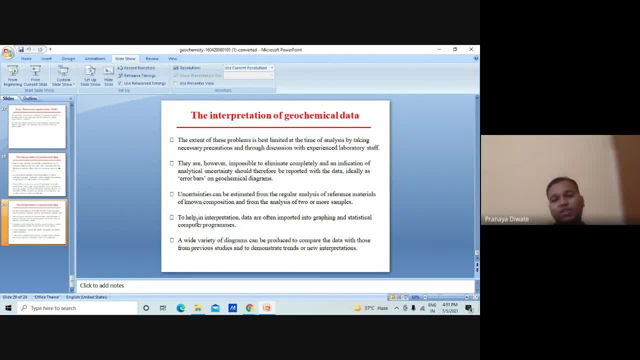 by studying the geochemistry, on all, by studying the geochemistry and all, uh, we are just uh, uh. so interpretation of this geochemical data is very, very uh, uh much that they. so the geochemical data is comparatively a very important data. or to know about the: what is the subset, what is the? 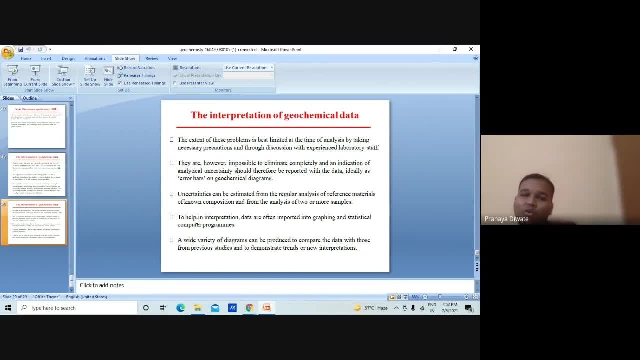 composition of same surface. you cannot go there. you cannot go there, so you need to take a in such a way that so the extent of the problem is, the geochemistry best fitted limited and the time of analysis by taking necessary precaution and through discuss with the experience on laboratory. 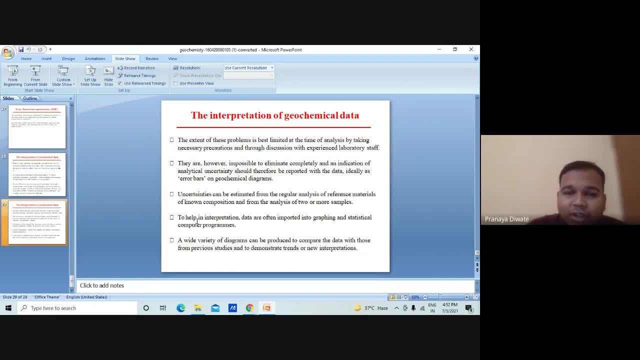 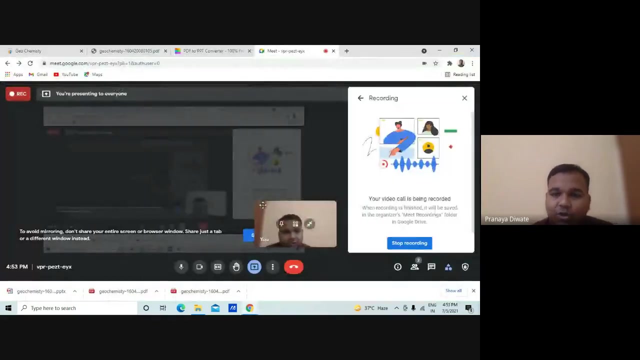 They are, however, impossible to claim on what we can say. So this is all about what we can say: the introduction to the geochemistry, introduction to the geochemistry. So what we learned today about the geochemistry, study of geochemistry. 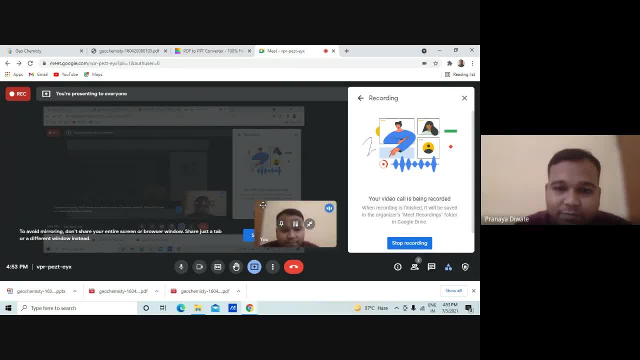 Study of this one. So you have what we can say the geochemistry as a subject. You can analyze this with the different instrument. You can learn those instrument and this one is very significant for you. Like, you have IRMS, so you can have a good number. 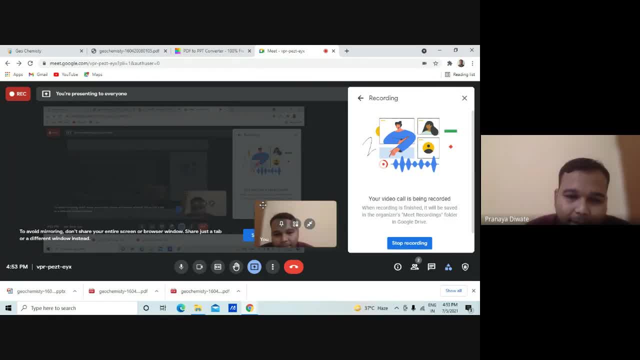 of jobs out there. So thank you. Thank you for listening to my video, this lecture. Whatever the engagement, these questions are there, So this is how you can have a different kind of scenario. Again, thank you for listening to this video. 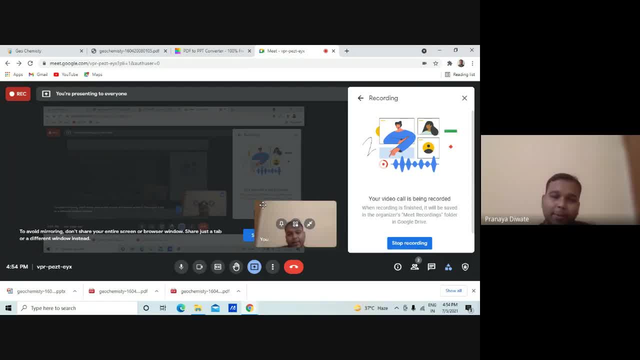 and hope you understand And so. So this is how you have a different kind of geochemical element And now in the next lecture we will also see about the sedimentary, What kind of processes have been that takes place for the hydrogeological groups.